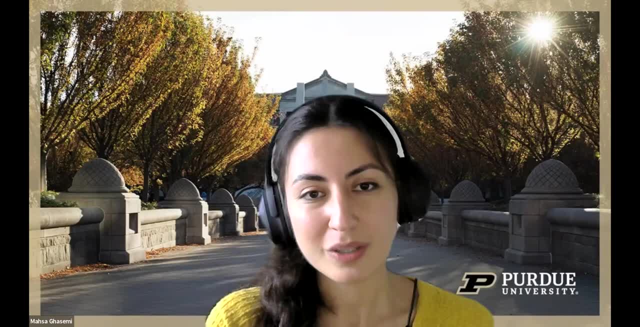 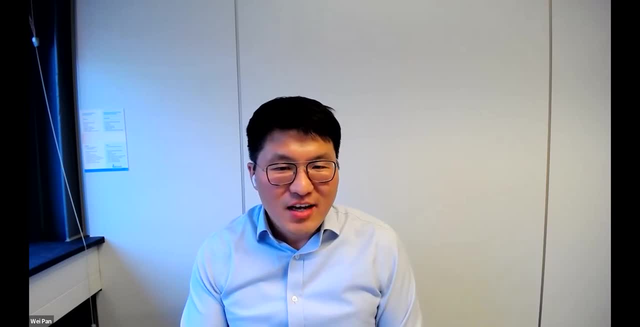 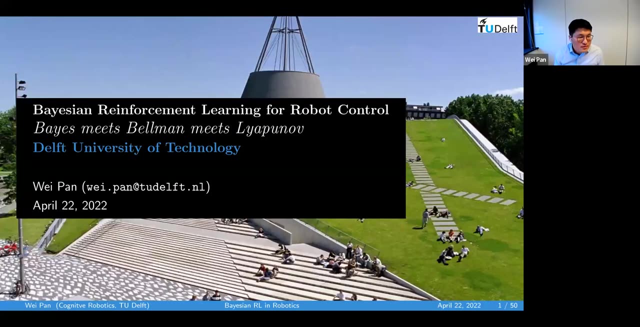 Automation Letters. So, without further ado, I invite Wei to start his talk. All right, thanks for the nice introduction and thanks to Xiaoshuai for the invitation. Okay, let me share my screen. Can you see my screen? Yes, 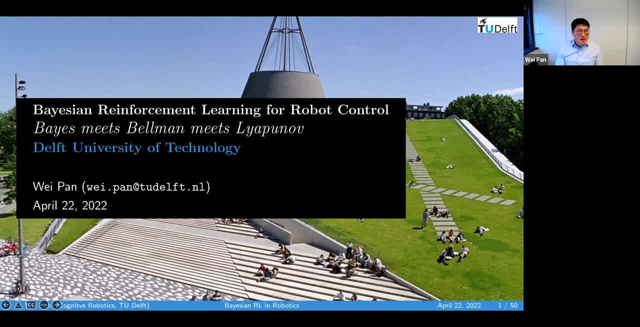 Okay, let me start. All right, good afternoon everyone, and thanks for the invitation And thanks, Marcia, for the nice introduction, And I'm currently in the Netherlands. Well, maybe I should say good evening to everyone, And my research is about control of robots And there 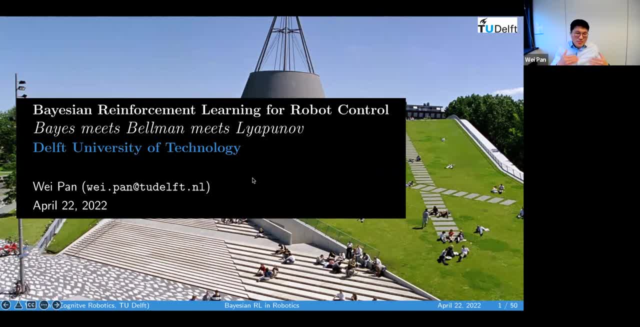 are quite some talks and works on reinforcement learning or deep reinforcement learning for robot control. Today, I'm going to talk about the Bayesian method of reinforcement learning for robot control. By using the Bayesian method, we can give safety-related guarantees, such as stability. 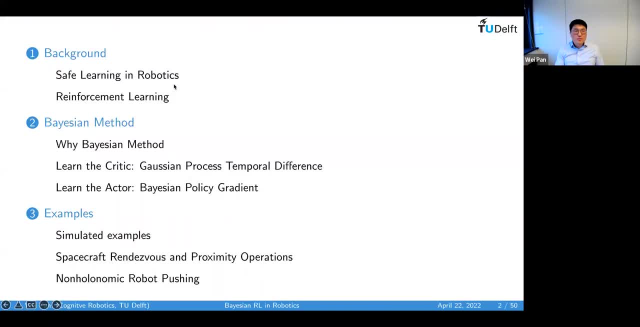 and some hard constraints guaranteed. Okay, here's the outline of my talk. First, I will give some background of safe learning in robotics and reinforcement learning, Then I will introduce the technical details of the Bayesian method And finally I will show some examples, including both simulation and real-world demos. 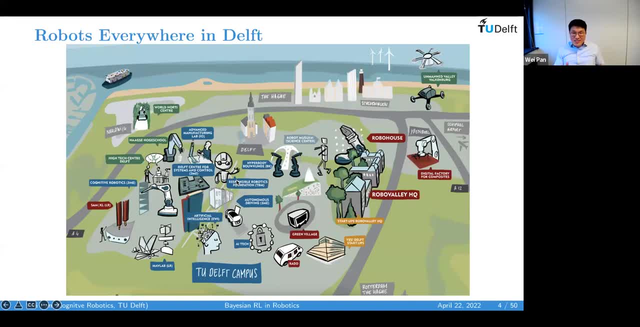 Okay, robots are everywhere in Delft in the Netherlands and the robotic research is every where in Delft. Robots are working for the people and working with people. For all these robotic applications, safety is crucial And for all these robotic applications we need to design reliable 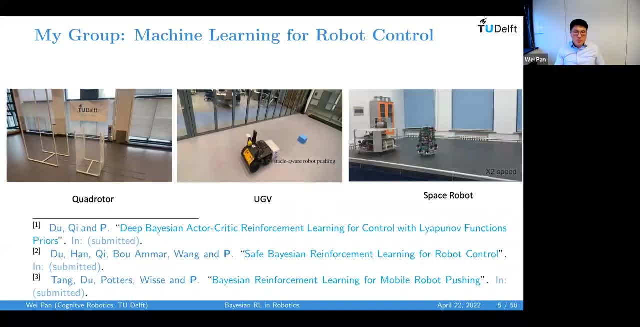 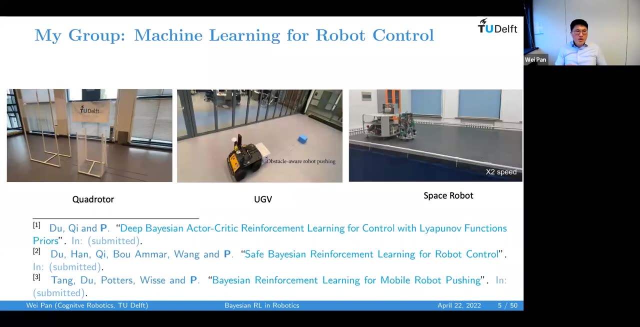 robot control systems, And my research group is focusing on machine learning for robot control. We work with different robots, for example, ground vehicles, drones and a space robot, And, for all the examples shown here, we are using Bayesian reinforcement learning to design robot controllers. 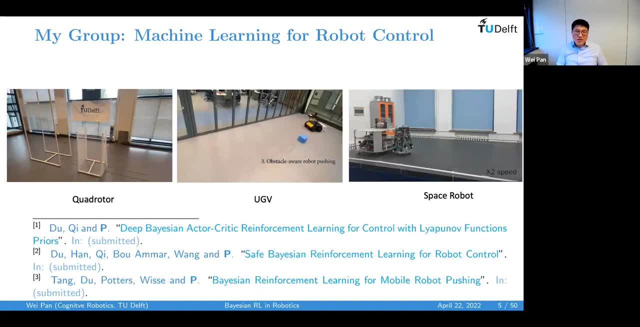 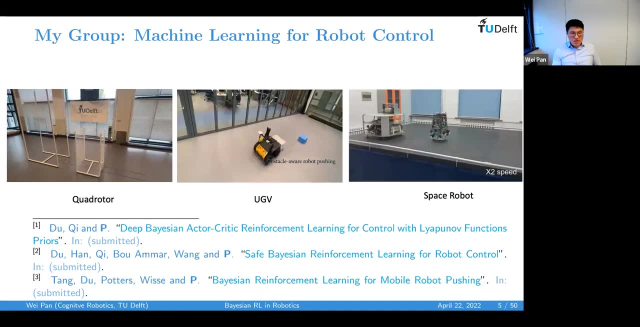 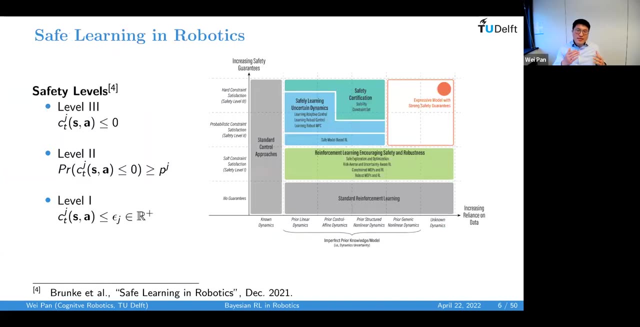 to ensure safety guarantees such as stability, collision avoidance and some other constraints. Today I will introduce some of our recent work on Bayesian reinforcement learning for robot control and with safety guarantee. Before I delve into the technical details, first I will give a quick 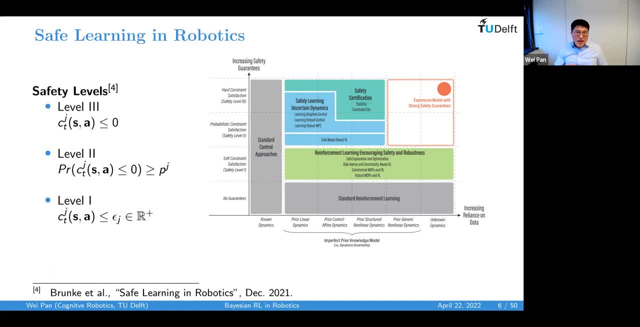 overview of safe learning in robotics. Recently, Angela's group from the University of Toronto published a review paper on safe learning in robotics. I agree very much with this paper And in this paper they define safety levels on three levels. So at the highest level, level three, the system. 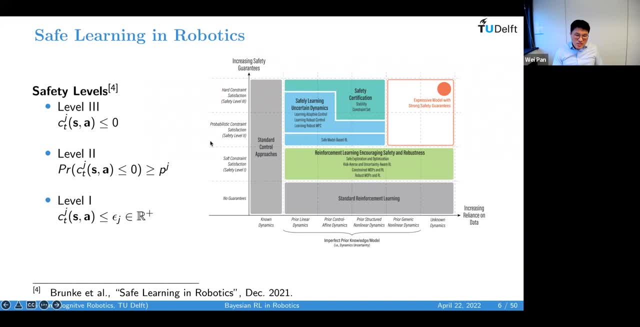 has to satisfy hard constraints And at level two the system has to satisfy probabilistic constraints And at the lowest level the systems are encouraged to solve the constraints. And also. this paper systematically reviewed approaches for safe learning control in robotics in several categories, highlighted with different colors here based on the complexity of the model. 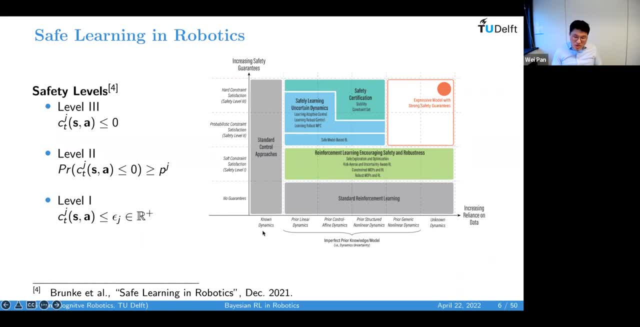 of prior knowledge about the system dynamics, from known dynamics to unknown dynamics, And it includes the standard control approaches which expand all the safety levels. It also includes the standard reinforcement learning method which basically there's no guarantee at all. We can move a little bit further to encourage safety and the robustness 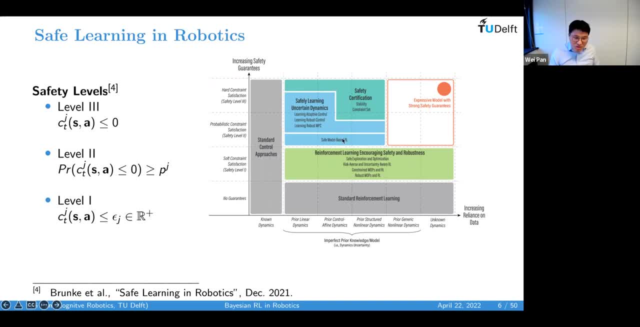 to reinforcement learning And we can move a little bit further more to safely learn the uncertain dynamics. And then in between we have the safe, model-based reinforcement learning At the highest level. the system can offer a safety certificate, including stability and a constraint set. 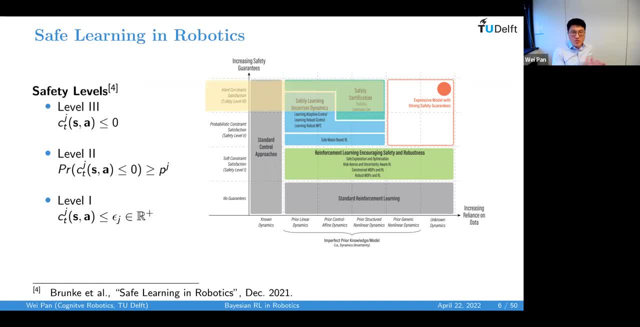 And today, in this talk, I will talk about safety and robustness. I will talk about safety and robustness. I will target safety level three- certifying learning-based control under dynamics and certainty, And I want to move closer to the final goal of certifying reinforcement learning. 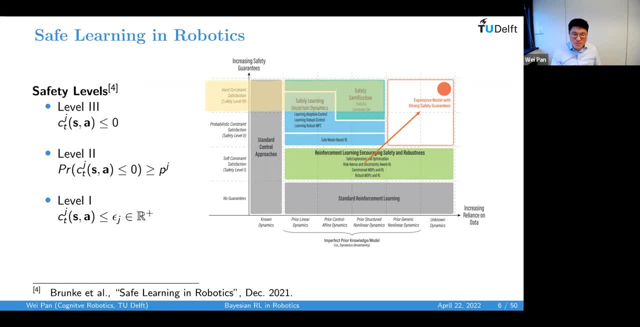 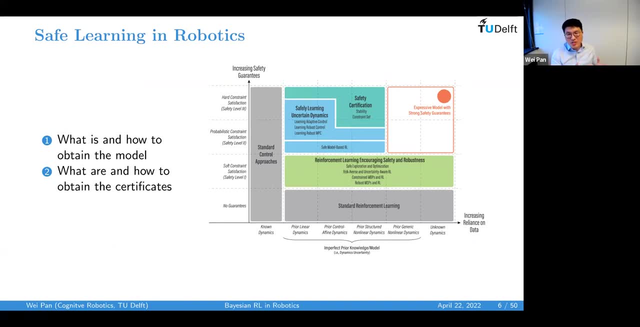 with these guarantees, either with or without using a mathematical model. Okay, Before presenting the theoretical result, we have to answer two set of questions, or maybe four questions here. So the first set of questions are: what is and how to obtain the 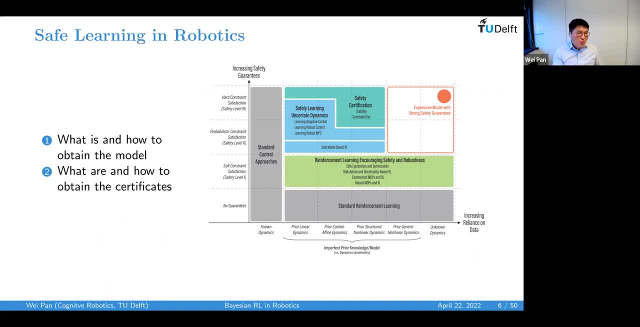 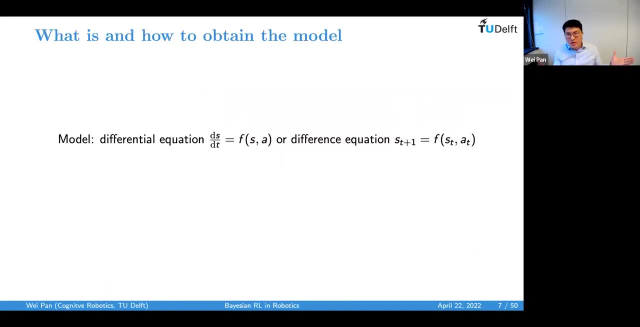 mathematical model. And the second set of questions are: what is and how to obtain the mathematical model? The second set of questions are: what are and how to obtain the certificates? Well, to answer the first set of questions, regarding the modeling, we need to know what. 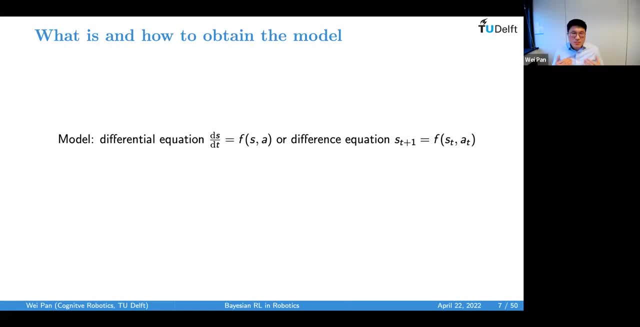 the model looks like. Typically, the system is modeled as a differential equation or difference equation. There are two ways of getting to the model. One is to use the first principle, for example, like Newton's law, to get a system equation. Well, the other way is to 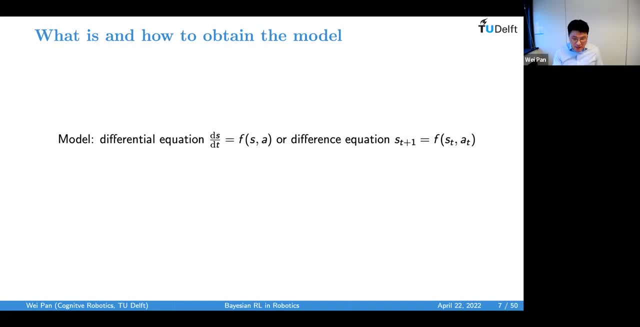 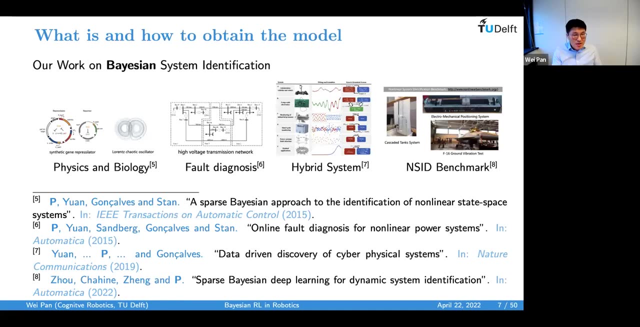 learn the model using some input and output data, known as system identification or model learning, And we have done some work on system identification by using the Bayesian method and applied it to different systems, For example from physics to anthropology, and also the fault diagnosis problem of high voltage transmission network. 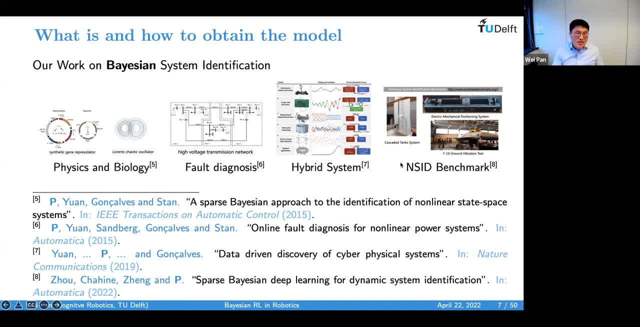 and some hybrid systems, as well as the nonlinear system identification benchmark. Well, it should be noted that this nonlinear system identification benchmark is a very popular in the Netherlands and the Belgium because, due to some historical reasons on the nonlinear system identification research here And our work on the Bayesian method of system, 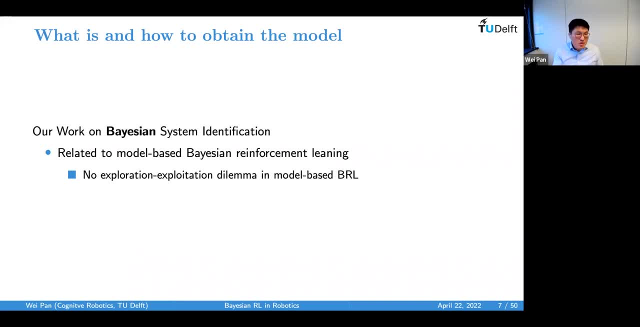 identification is related to the model-based Bayesian reinforcement learning. Well, you can use the uncertainty of the parameter to update the policy search in order to find the optimal policy, try to balance or compromise the exploration and exploitation. so there's no such dilemma in the model-based Bayesian reinforcement learning. However, I will not talk about the 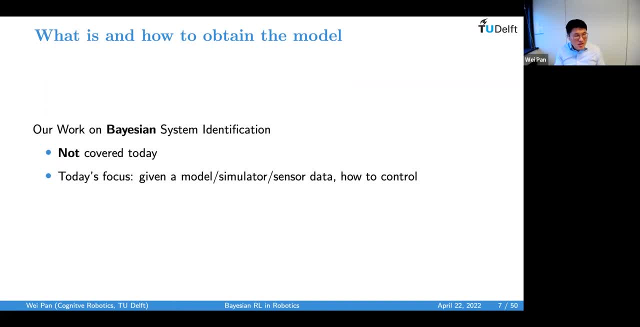 system identification today. Today I want to focus- if we are given a model, a simulator or just some raw sensor data, how to control the system. Now we have answered the first set of questions regarding modeling. right, Let's answer the second set of questions. What are, and? 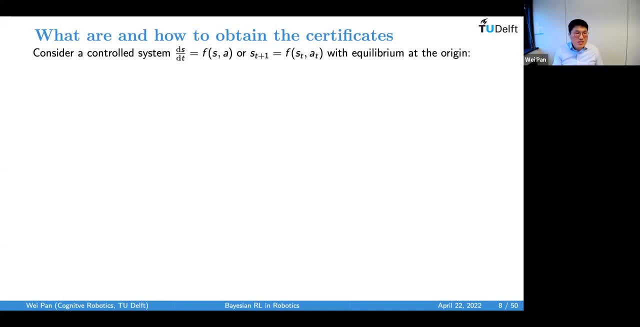 how to obtain the certificate. Typically, we are given the system by a differential equation or equation with the equilibrium at origin, and we can offer stability certificate. Typically, we are using Lyapunov function, which is a scalar function and a positive, and we hope that the 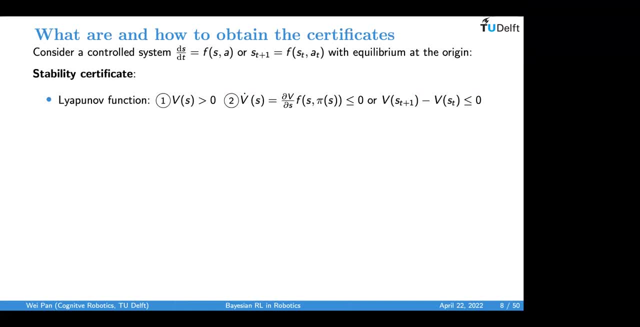 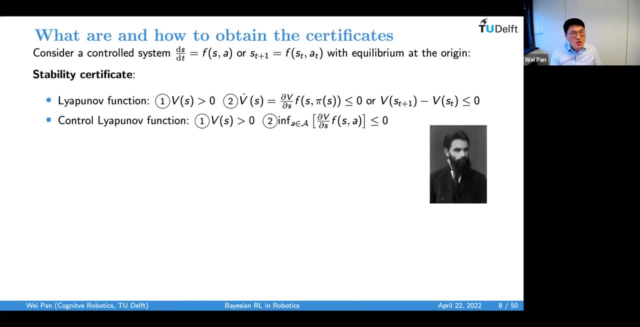 derivative of the Lyapunov function over time is non-positive, and also the difference is non-positive for discrete time system And similarly we can have the control Lyapunov function. Well, you don't have to define explicitly the feedback control law, You can just evaluate. 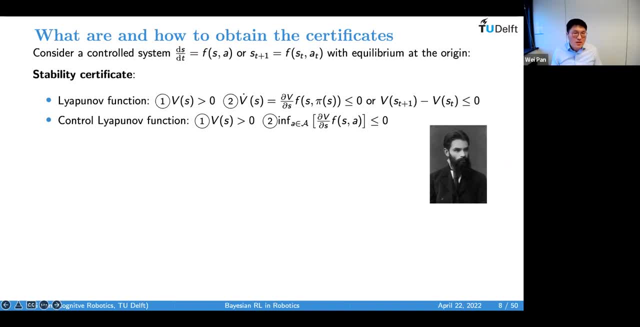 the actions And we make sure this derivative over time is non-positive And furthermore, we can have the safety certificate by using the barrier functions. So the barrier functions is also a scalar function and for some initial safe state so this barrier function is non-positive and for some unsafe. 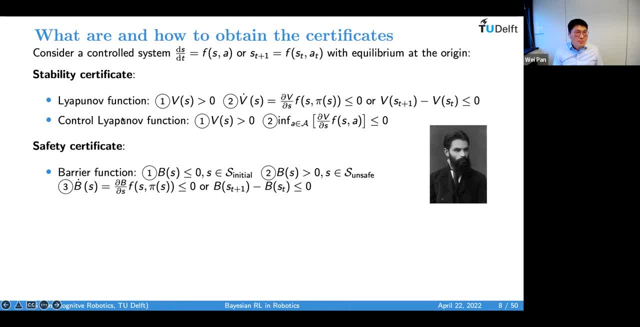 regions. the barrier function is a positive and similar to the Lyapunov function. the derivative of the barrier function over time is positive or with the difference is non-positive- sorry. And similar to the control Lyapunov barrier function. we can have the. 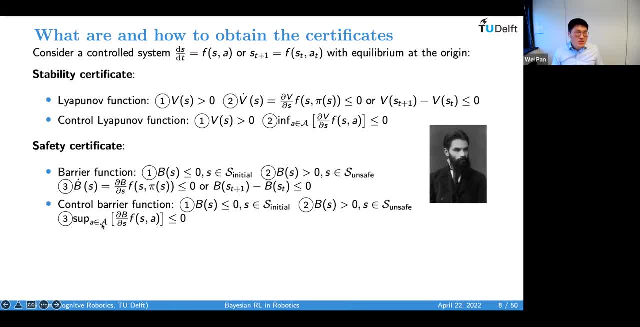 control barrier function and we are evaluating the actions and make sure this derivative is non-positive. We can also unify the stability and the safety certificate and get the control Lyapunov barrier function, which is the positive scalar function and in some safe regions. 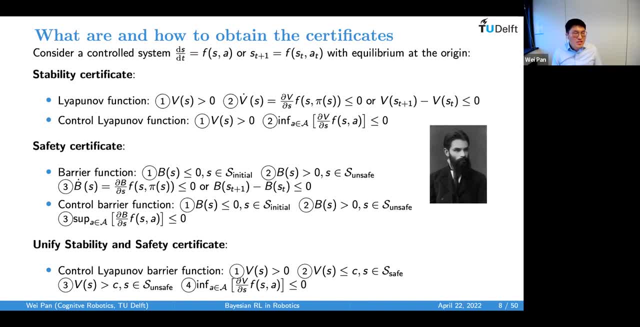 it's smaller, equal than c, some constant, and when it's in the unsafe region, it's greater than c. and then we evaluate the actions and make sure the derivative is is non-positive. Well, what I introduced here is just a nutshell and it may be oversimplified or even not rigorous. 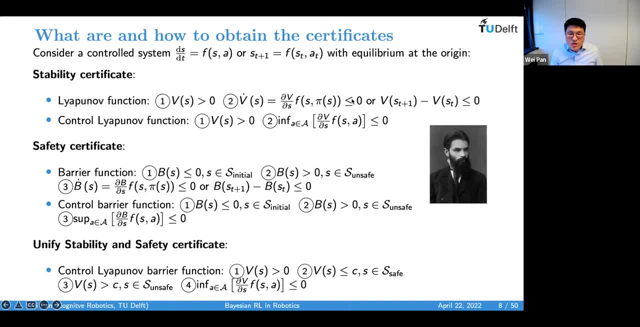 For example in the Lyapunov function case for the zero it often substituted by a minus class kappa function, And the zero here for the Bellary function is often substituted with the minus extended plus kappa infinity function. So the idea I want to show here is that 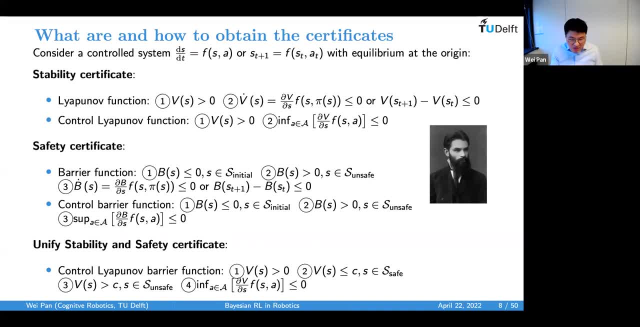 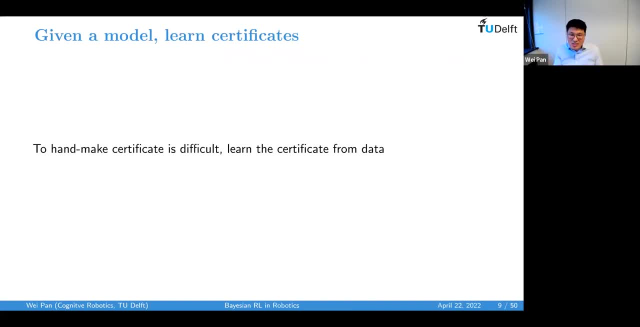 the safety related certificates are kind of a bunch of inequalities. Okay, now we know what are the certificates. then how to get these certificates? Well, unfortunately you have to handmade your certificate. It is notoriously known that it's very difficult And luckily and recently, there are some work. 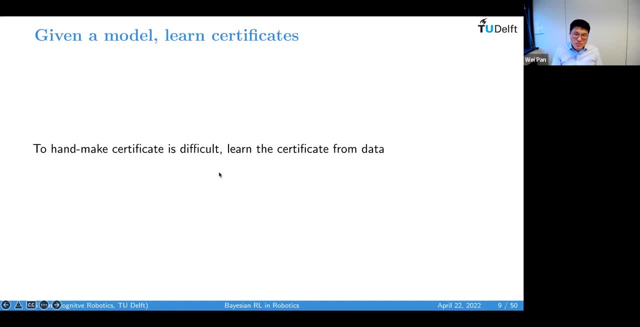 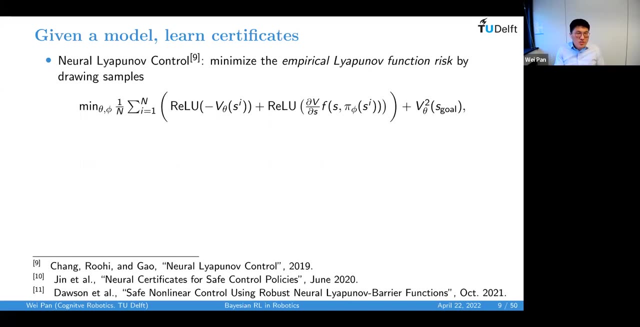 showing you that you can actually learn the certificate from data if we are given the mathematical model okay. For example, like in this case, you're in the Lyapunov control. the authors are trying to tell you to try to minimize the empirical Lyapunov function risk. 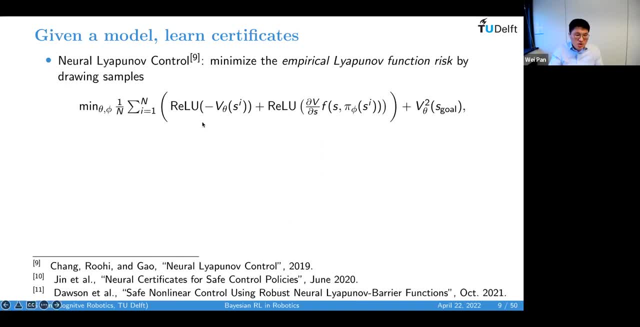 by drawing some samples. So the right-loop function here is to showing or drawing the connections between the constraints in the equalities And in this paper, actually from Xiaoshuai, and they are trying to combine the Lyapunov function and the Bellary function by minimizing the Lyapunov-like risk. 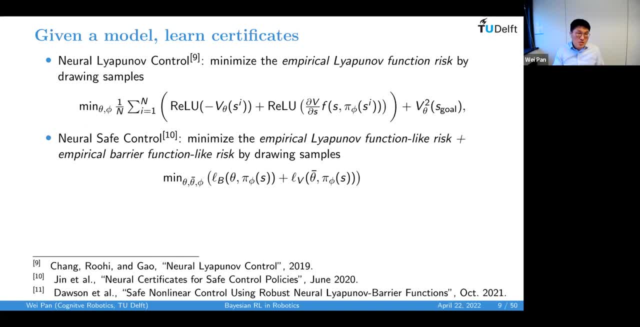 and the Bellary function-like risk and drawing samples, and about also using the right-loop functions to transform the inequalities of the inequalities into the certificate in the cost of function. And in this paper they are trying to combine or propose a unified control Lyapunov-Bellary function. 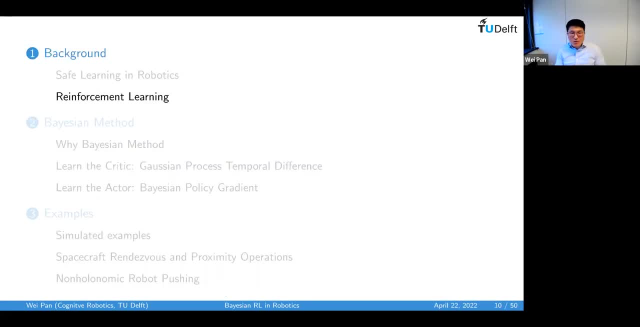 and by drawing samples. Until now, we always assume we have a mathematical model of the system. What if we have unknown dynamics? For example, we're just given a simulator or just some raw sensor data. How to do that? How to design the controller? 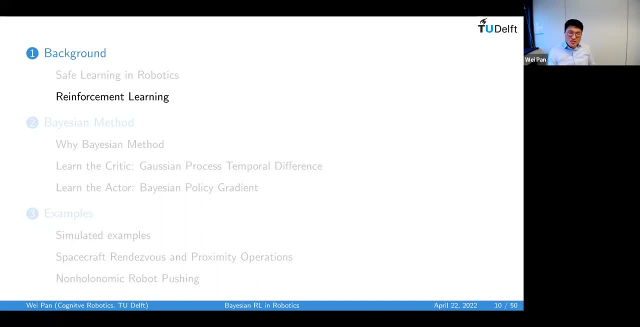 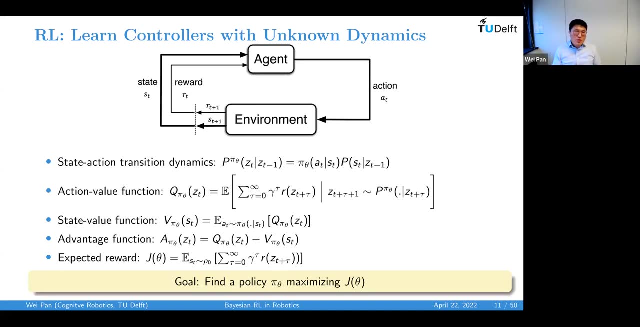 Well, reinforcement learning is a promising approach To learn controllers with unknown dynamics from data. So what is reinforcement learning? Well, in the reinforcement learning framework, there's an agent, there's an environment. Well, the environment can be the robot. 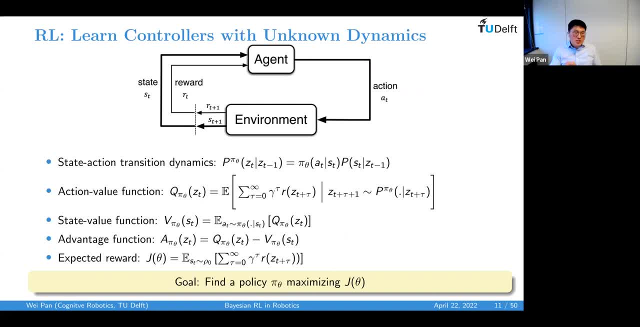 And the environments are interacting with the agent And through such interactions the agents begin to learn the policy which is optimal to control the environment. And typically the environment is modeled as a markup decision process or some partial observable markup decision process, and so on and so forth. 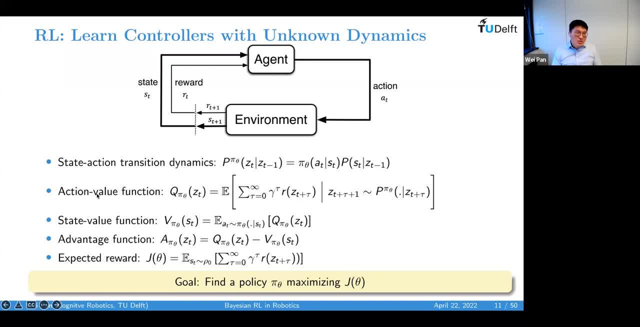 And we have the state action transition And we have the action value function Q, which is an expectation of the sum of the discounted reward for the future, And we have the state value function, which is the expectation of this Q function over some actions, which is sampled from policy pi. 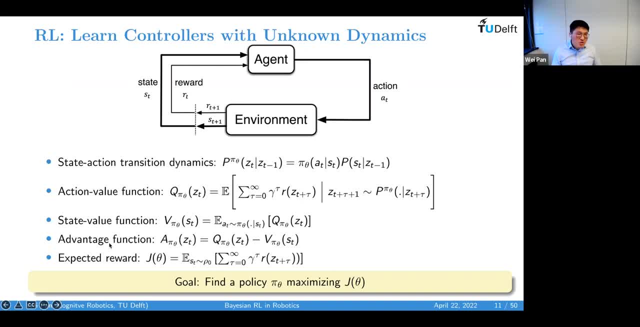 And we have the advantage function, which is the difference of the action value function Q and state value function V. And we have our objective, which is expected reward, And our goal is to find a policy pi which can be promised by some parameter, theta. 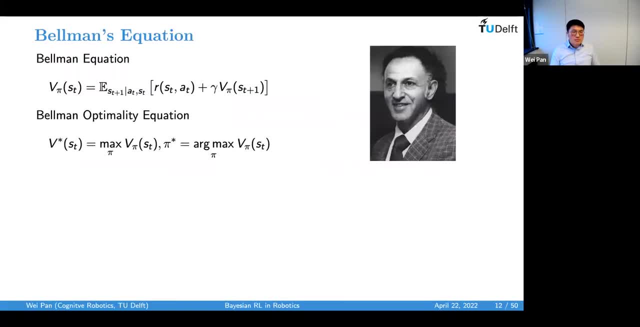 to maximize our objective, the expected reward. How to solve the reinforcement learning problem? We can rewrite the objective function as the Bellman equations and use the dynamic programming. We can derive the optimal policy using the Bellman optimality equation, typically using the like value iteration. 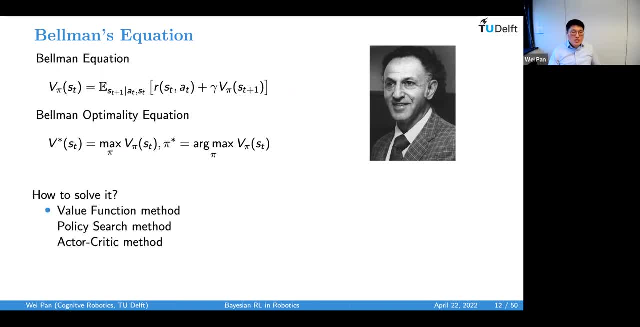 algorithms or policy iteration algorithms. Well, these methods are value function-based methods. An alternative approach for solving MDP is to directly search in the space of policies. Or you can combine the value function method and the policy search method and came up with the actor-critic method, while you simultaneously 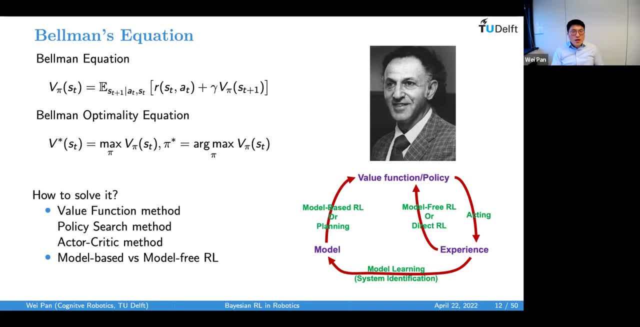 learn the value, function and the policy. Besides the category of the reinforcement learning solutions by the algorithms, the other category is based on the use of the model. Typically in the model-based RL, the model is not available, but it is explicitly learned from experience using some model learning or system. 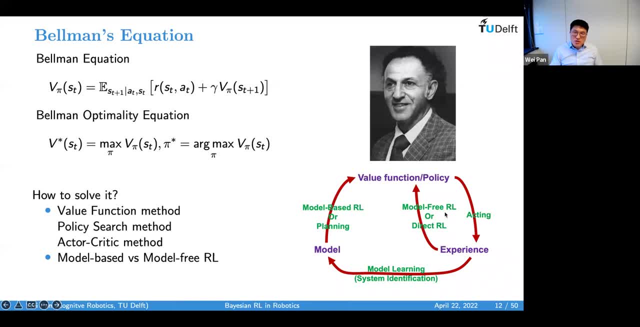 identification techniques. Then the model will be used for planning, Then interacting with the environment through some actions to collect more samples, to update the model And in model-free reinforcement learning. the model is not available and is not explicitly learned Through actions with the environment and the value. 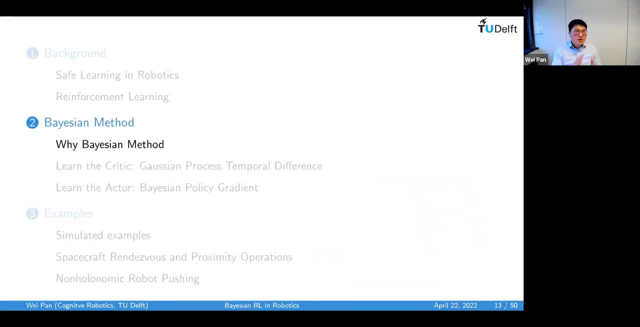 function and the policy will be learned. Why am I talking about a Bayesian method of reinforcement learning? You can just use the vanilla reinforcement learning to control robots And there are so many videos, demos and interesting applications just using the reinforcement learning per se. 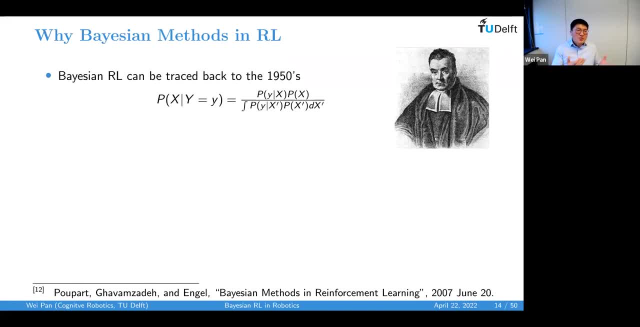 not using the Bayesian method? Well, Bayesian reinforcement learning is very old. It can be traced back to the 1950s. Well, this is typically known as the posterior. This is the prior, This is the likelihood, And this integral is a normal factor. 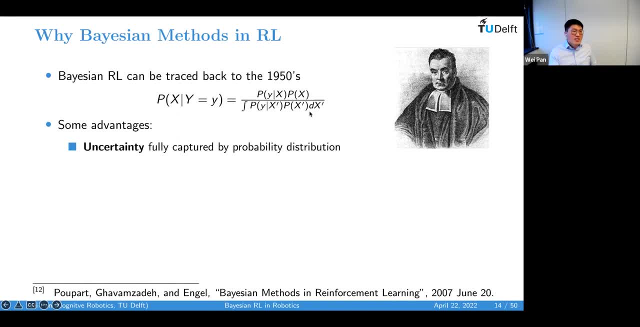 or known as the evidence. Well, indeed, it has some advantages. Well, the uncertainty can be fully captured by the probability distribution And this is the natural optimization of the exploration and exploitation trade-offs. And it is also a unifying framework for other learning frameworks. 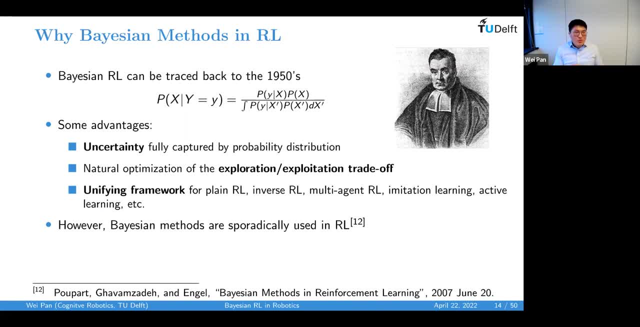 However, still the Bayesian methods are rarely used and that we barely heard any applications. I mean real world applications, especially in robotics using Bayesian reinforcement learning. Well, in my perspective, I think the challenge is there's no guidelines to place priors on what 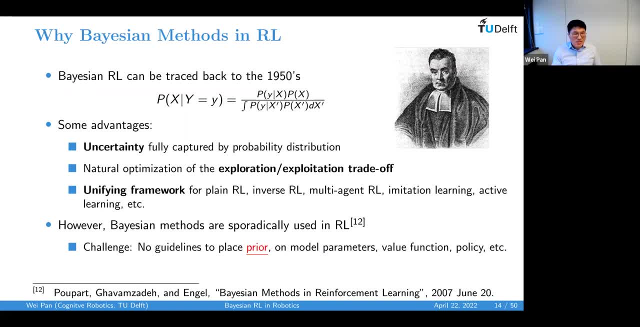 On the model parameters, value functions or the policies. Well, challenge also means opportunity, right? Maybe we can have some good domain knowledge, for example, in the certificate to place priors on the value functions. Why not? Let's do that. 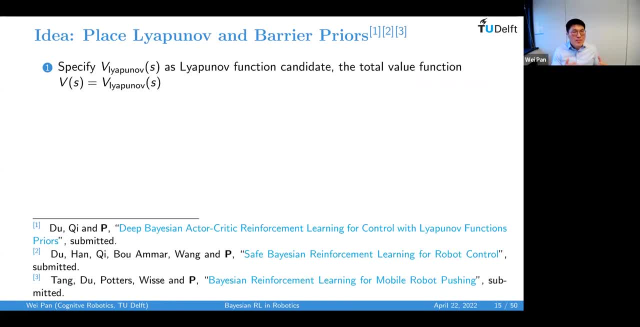 So the idea is that I want to place Lyapunov function and the barrier function as priors. OK, first of all, we're going to specify the value function to be the Lyapunov function candidate And furthermore, if we care about the safety, 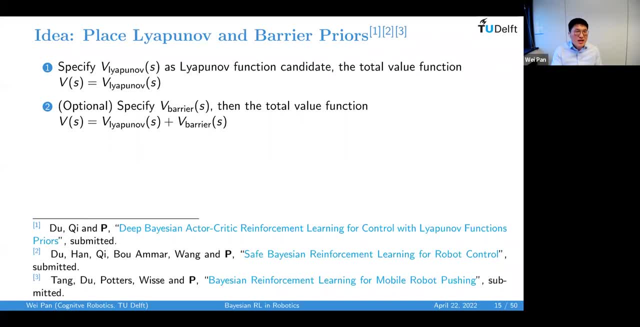 you can specify the barrier function as this And then the total value function is going to be the sum of the Lyapunov function and the barrier function. Then we can write a bunch of inequalities as we can see in the certificate as a prior distribution to encode the distribution. 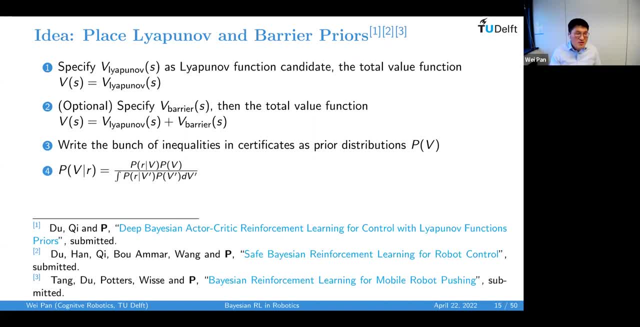 of the value function right, Then we can use the Bayesian inference approach to get an estimate of this value function. And finally, if we can find a way to get a cue from V, then we can apply the policy search to get the optimal policy. 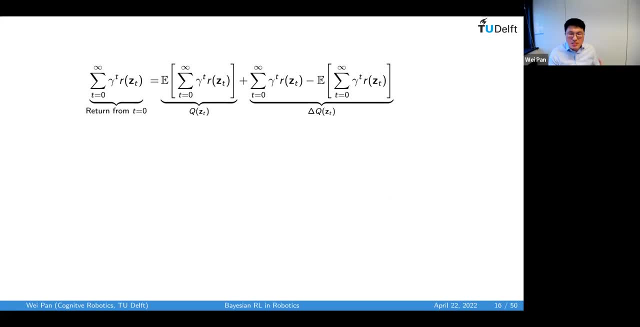 Well, how can we do that? We can decompose our objective, the sum of the discounted reward, as follows: starting from T equals zero. And furthermore, we decompose again starting from T equals one. Then we do the subtraction on the left-hand side. 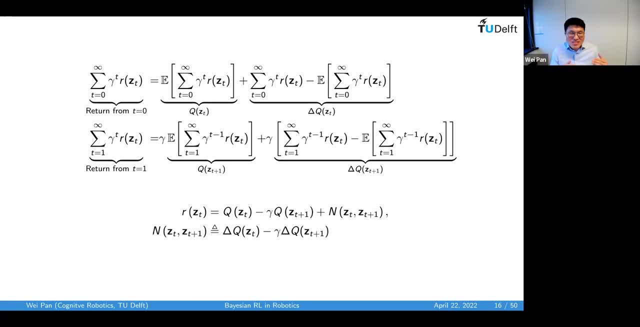 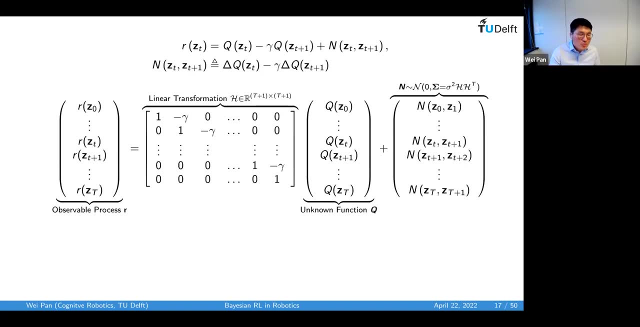 and the right-hand side, we get the following equation: Well, this is essentially temporal difference learning, And we can extend in a matrix form. We have the following representation On the left-hand side is the observable process of the reward, And then we have the linear transformation matrix. 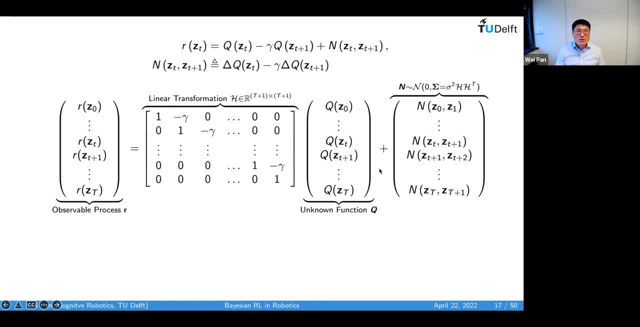 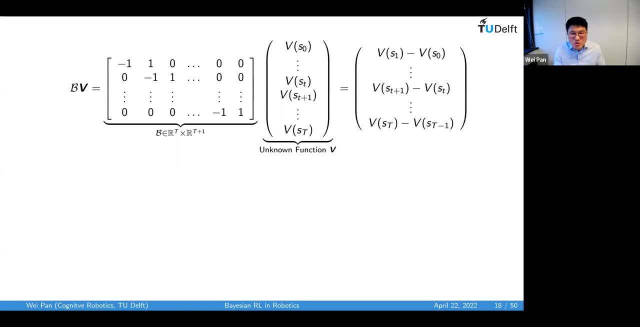 and then we have the unknown function Q, and then we have some noise. Then this is regression problem, right? So we can solve that. Let's do something further by introducing the B matrix, which is called the first-order difference equation or first-order difference matrix. 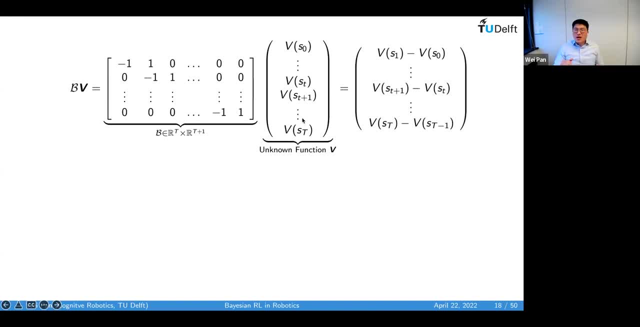 over the value function V. If we on the right-hand side it is the time derivative, It's a time difference of V over time, Since we haven't specified the state value function as the linear function candidate, if this right-hand side is not positive, 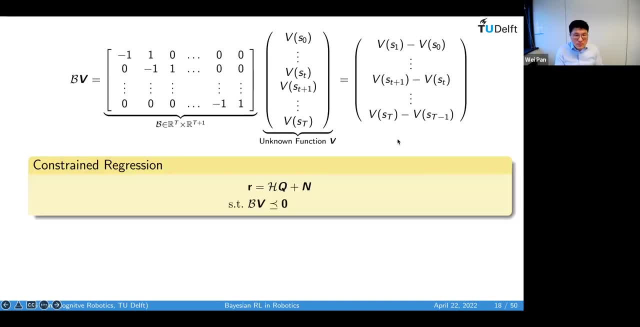 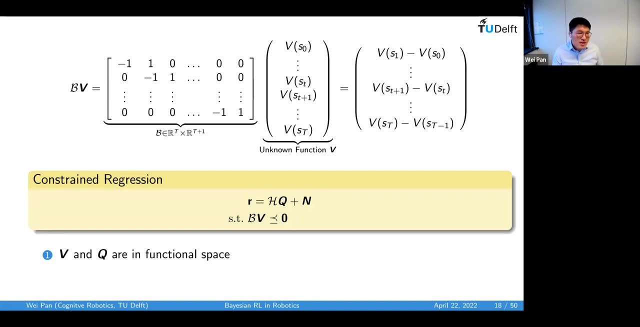 we actually have the stability certificate, Then we can have the constraints regression problem formulation. If we can solve both Q and the V, we are done. However, there are two problems. The first problem is: V and Q are in the functional space. 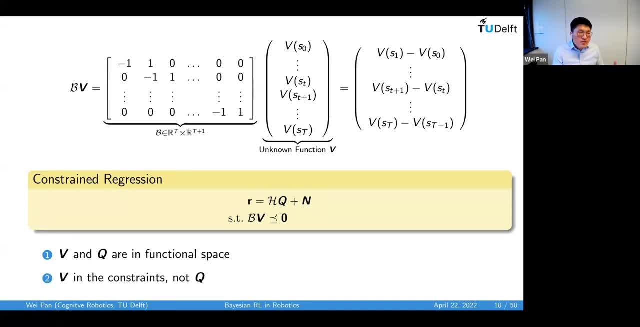 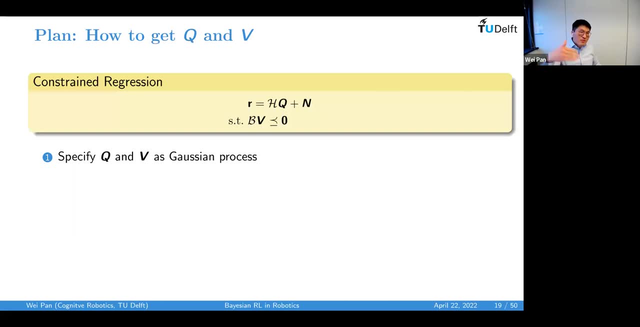 It is not just a number, right, And the V is in the constraint, Well, not Q. And how to solve these problems? Well, let's make another round of the plan. We specify Q and the V as Gaussian process, And if we can easily derive Q from V, 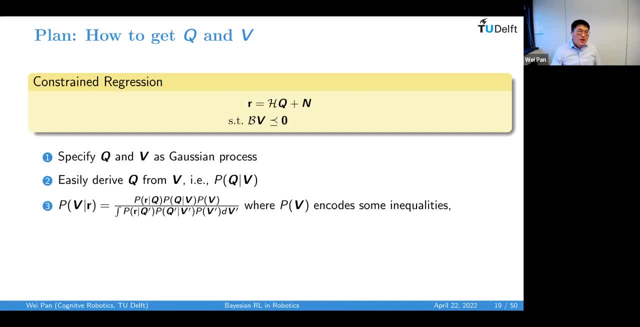 that is the probability distribution of Q condition on V. then we can use the Bayesian inference where PV encodes the sum of the inequalities. then we can get the certificate. If we get a Q, we can use the policy search to search the optimal policy. 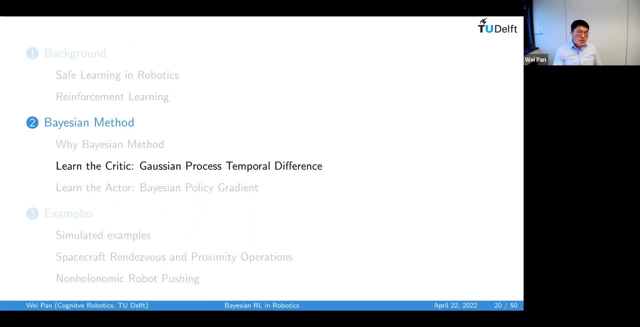 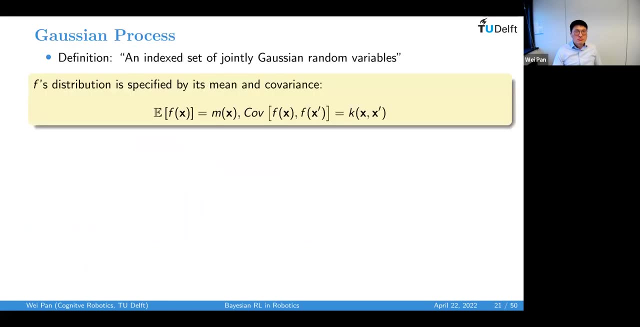 Okay, So we're going to use the actor critic to learn: the critic by using the Gaussian process- temporal difference- and the learned actor using Bayesian policy gradient. So what is the Gaussian process? So the Gaussian process definition is: there's an index set of joint Gaussian random variables. 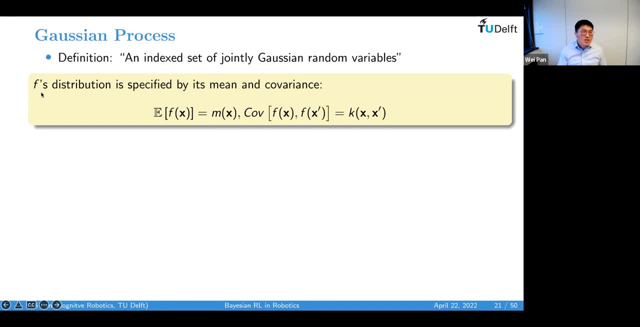 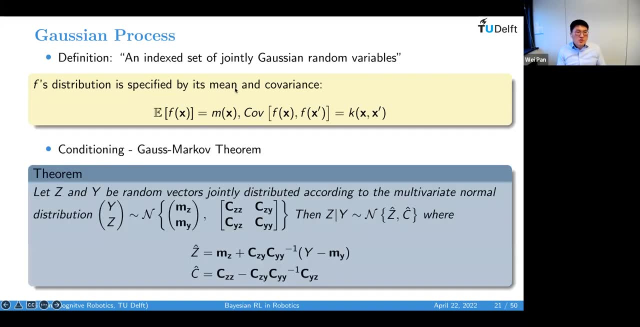 Suppose we have some input data X, we have an unknown function F, So F distribution is specified by its mean and the covariance And we can also use the conditional probability. Suppose we have two random variables jointly distributed according to the multiple variety normal distribution. 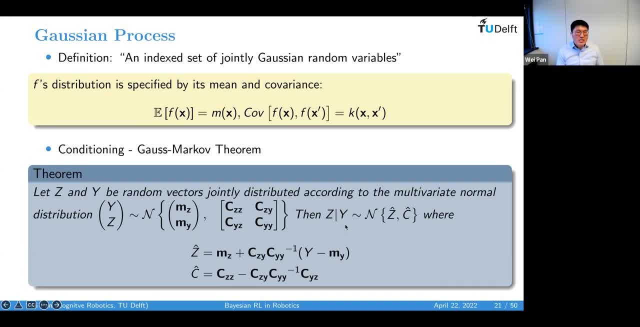 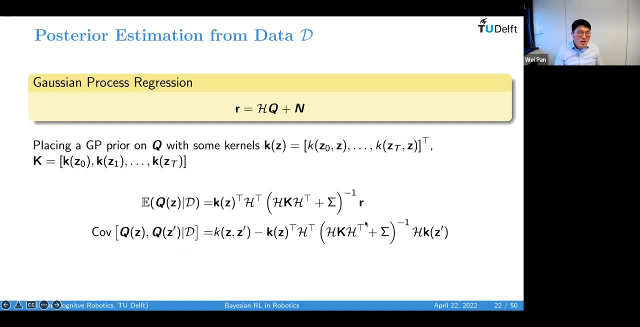 we can derive the conditional distribution of Z over Y as follows, which is also Gaussian. Then we can easily solve the regression problem by placing a Gaussian process prior over Q. Okay, So far, just pay attention, There's no constraint yet. Then we can solve that easily. 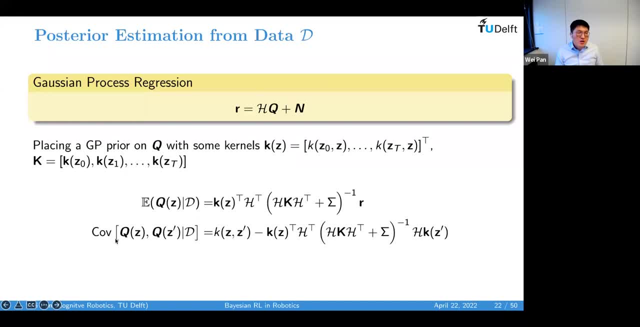 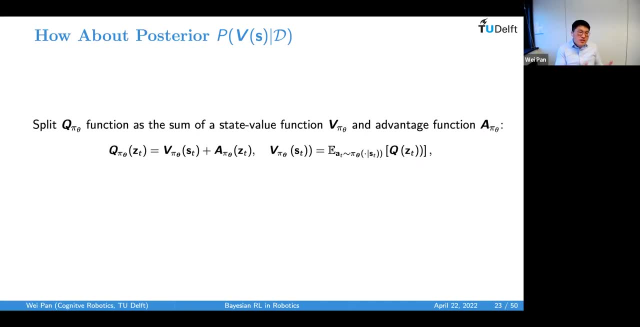 by deriving the posterior estimation of the expectation and the covariance as follows. Furthermore, how about we get the distribution of V over the data? We can split the Q function at the sum of the state value function V and the advantage function A. Then we can denote this variable here. 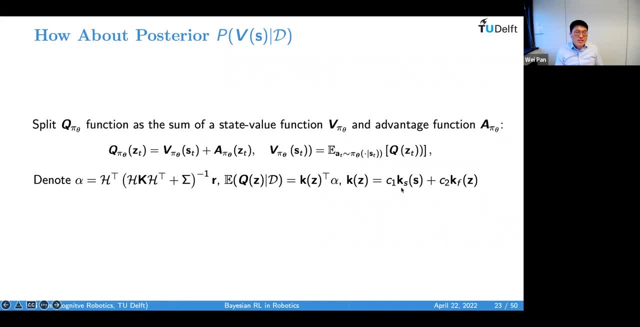 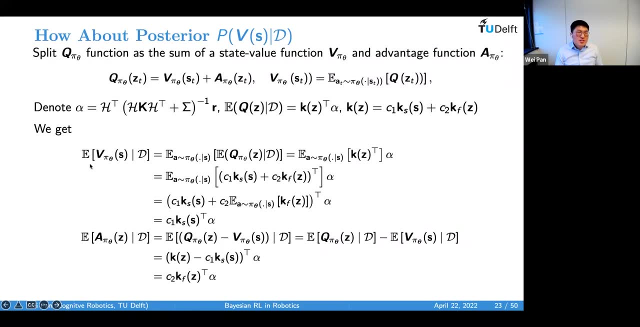 And by selecting such a kernel, which is the sum of the sum state kernel and the sum state action kernel, by some derivations we can find that, okay, the expectation of V over D is actually corresponding to this state kernel, While the advantage function is only corresponding. 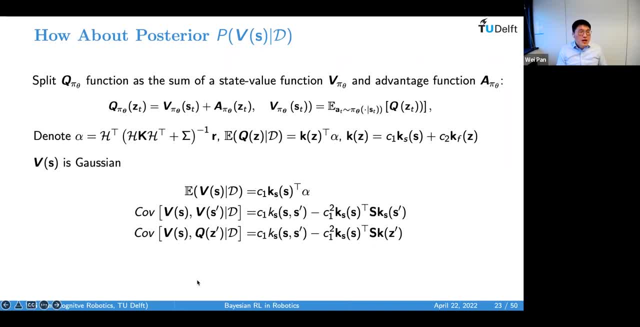 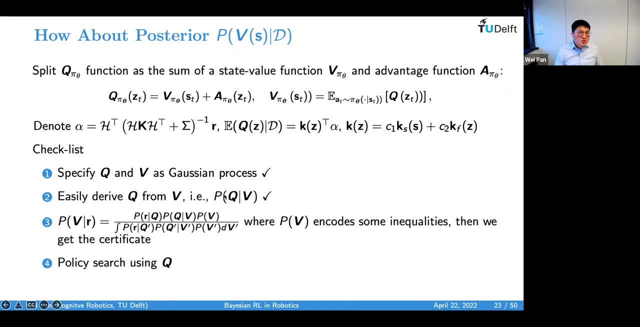 to the state action kernel. So V is also Gaussian And we can easily derive the covariance and the covariance of V with Q besides the expectation Right. Then we can easily derive Q from V, So we have the probability distribution of Q over V. 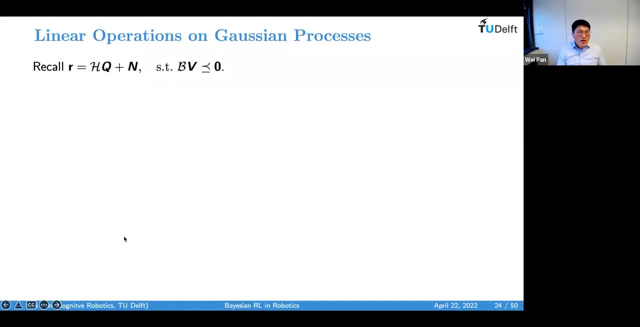 Now let's move to the next step. Recall that we want to solve this constraint regression problem, or the Gaussian process, or the constraint, the Gaussian process, regression problem. So actually, instead of putting a prior over V, we should consider BV. B is the first order difference matrix. 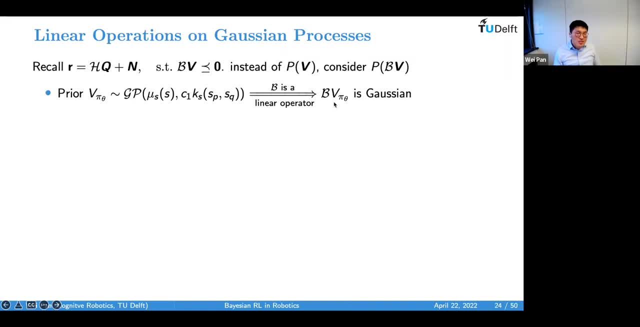 And if we specify this prior and with: B is a linear operator, so the BV is also Gaussian, then we can easily get the mean and the covariance and also get a cross covariance as follows: So now the idea is that if you consider the constraint case, 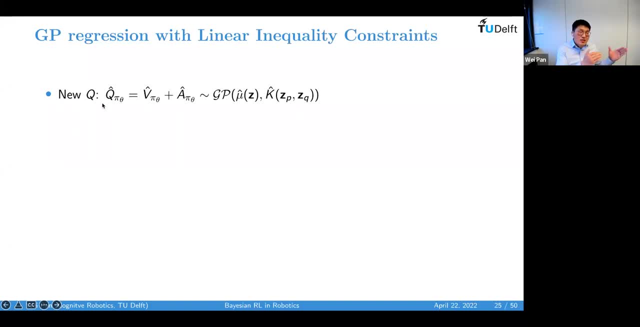 so we have a new Q besides the constraint, unconstraint case right. So with these linear equality constraints and also define CD, denote the event that all the constraints satisfied, the posterior Gaussian distribution conditional on the data side reward and this constraint event. 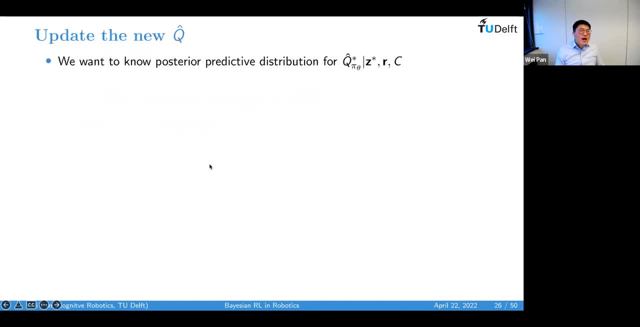 can be described as follows. Then our idea is that and our objective is we want to update this new Q hat, We want to know the posterior distribution for Q hat with some new state action pair. So the Q hat it's actually a compound Gaussian. 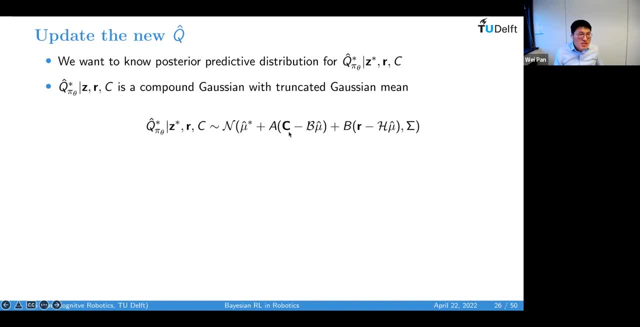 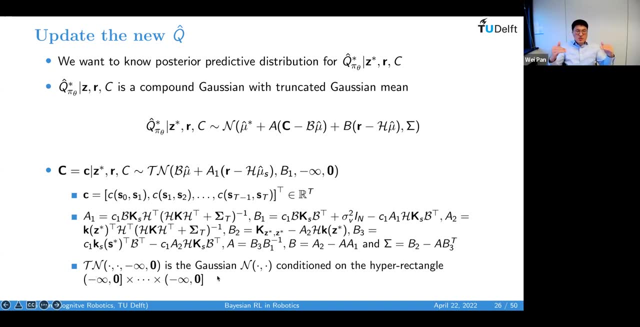 with the truncated Gaussian mean. So that's the key here. So C is actually a truncated distribution. So what is truncated Gaussian distribution? It's like you have a Gaussian distribution right, So in this case you only care about the negative part. 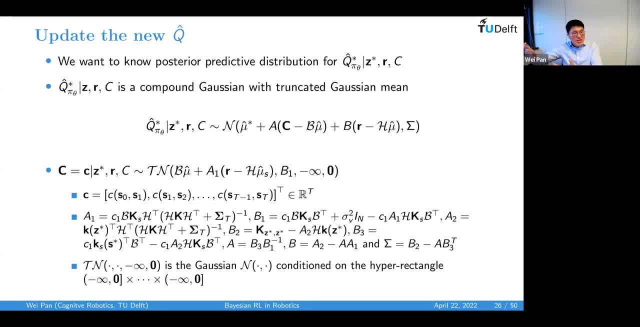 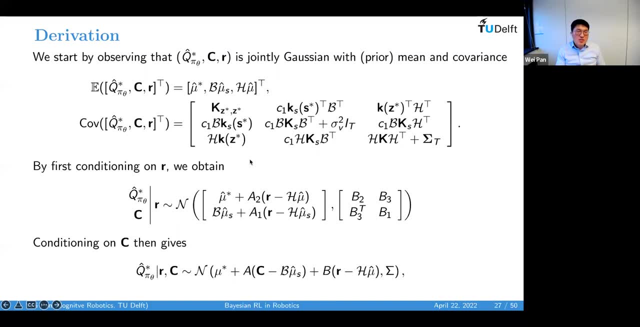 You only care about the left-hand side without considering the right-hand side of this Gaussian distribution. All right, And by some derivations we are repeatedly using the conditional distribution as follows: that we can get the conditional, we can get the Q hat. 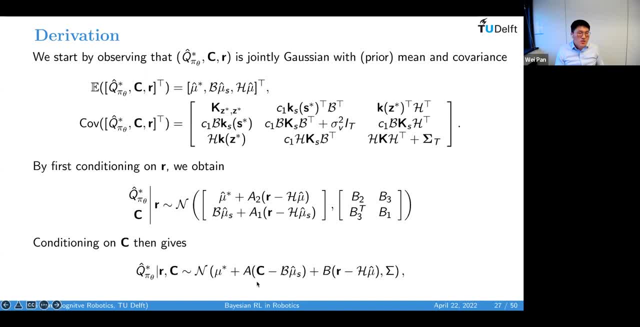 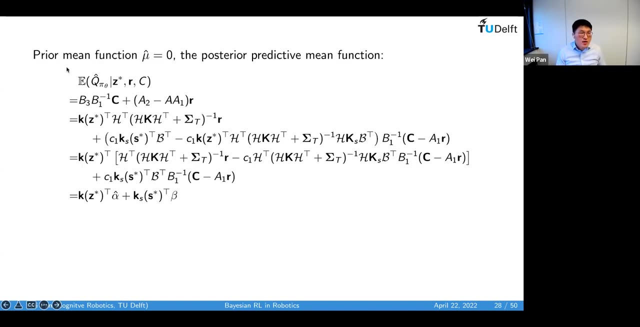 the Q hat conditional on C and the reward as follows: And the C is the truncated Gaussian distribution. So we can see that, we can see that this new Q hat has a truncated Gaussian distribution mean, All right, And we have, if we have, a prior mean. 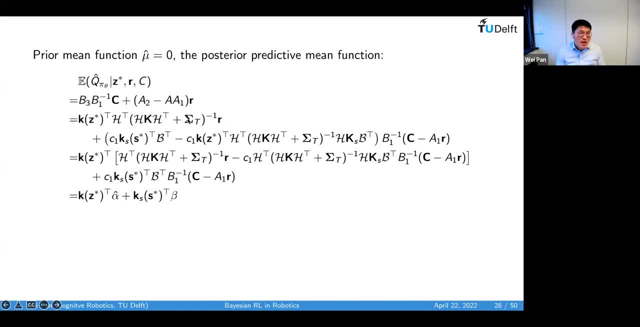 mu hat at zero, so we can have the posterior, predict the mean function and as follows. And if you remember that we have an alpha here for this unconstrained case, So in this case we have the new alpha hat here. So this is alpha minus something. 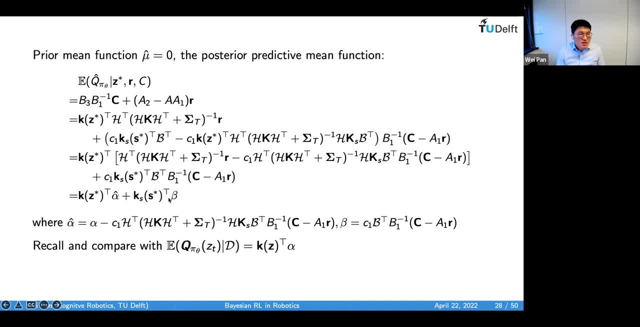 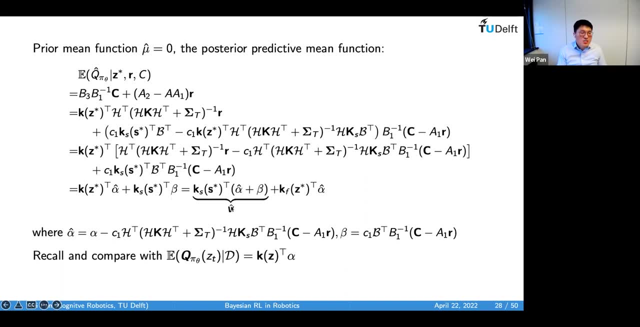 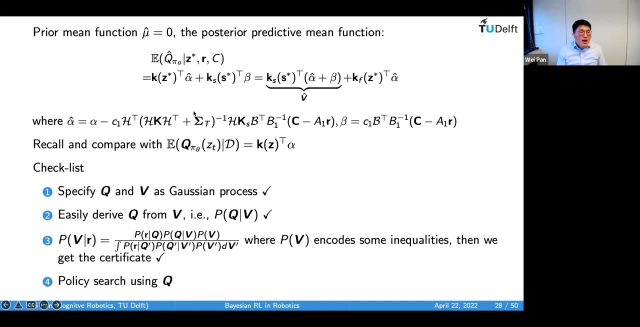 minus some truncated Gaussian distribution, plus some state kernels multiply the B And furthermore, this is actually only depends on the state kernel. So this is new V hat And this is our Lyapunov function And so far we can say that. 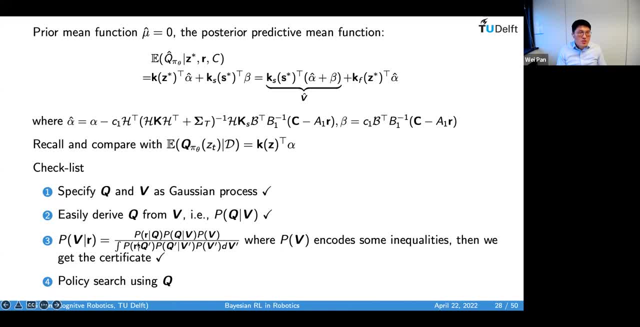 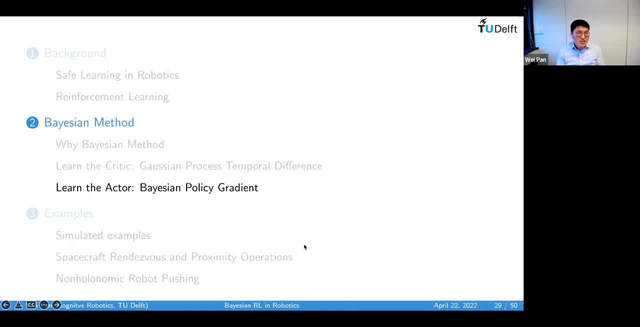 okay, we can do the Bayesian inference to get this V. Okay, Let's move forward to learn the actor, to learn the policy by using the Bayesian policy gradient. If we are doing a policy gradient, we definitely should show the policy gradient theorem. 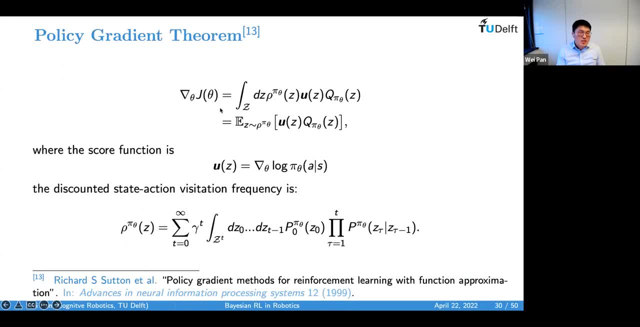 which is very famous. So basically, the policy gradient is expectation of this U multiplied the Q. So the U is the skull function with this gradient of a log pi And the Q is just what we learned from the critic. right Now we can use the Monte Carlo estimation. 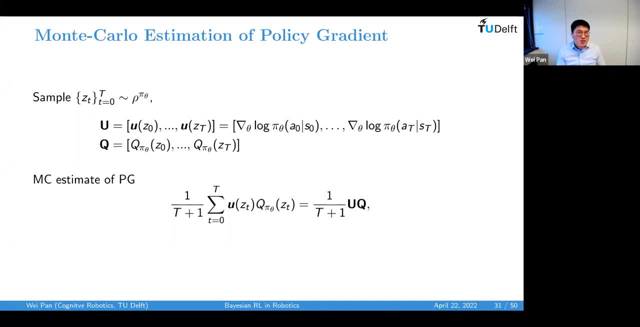 to estimate the policy gradient, So simply by simply drawing some samples. However, there's a problem with the Monte Carlo estimation method because the variance is very high by doing the Monte Carlo simulation, Since we have specified the Q as a Gaussian process and actually there's an opportunity. 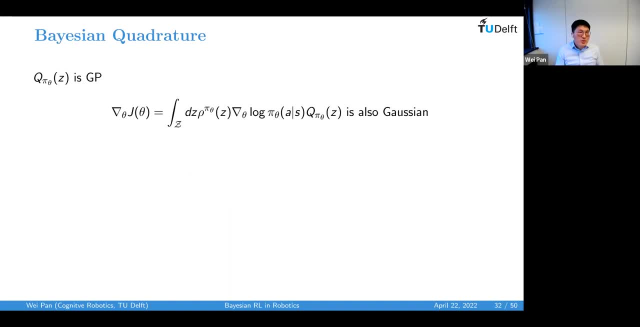 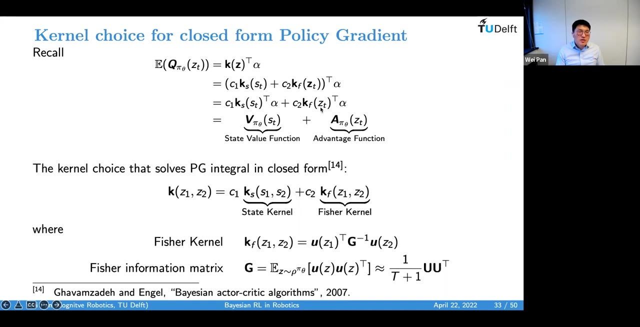 we can get a close form of the policy gradient by using the Bayesian quadrature And we can simply derive the posterior moment as follows: Recall that we construct the kernel function at the sum of the state kernels plus some state action kernels, right. So if the state action kernel 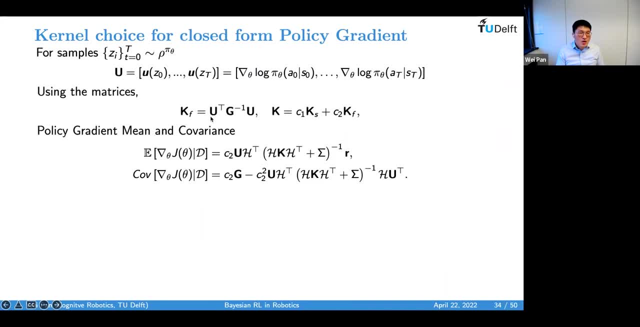 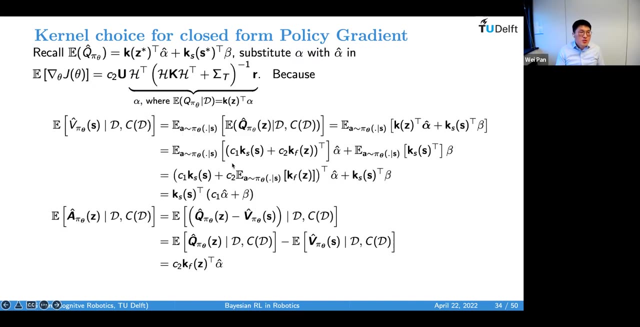 is specified as a Fisher kernel, then we can get a close form solution for the expectation of the policy gradient and the covariance as follows. And if you remember this alpha is in the constraint case. then we can say if we are using the constraint case. 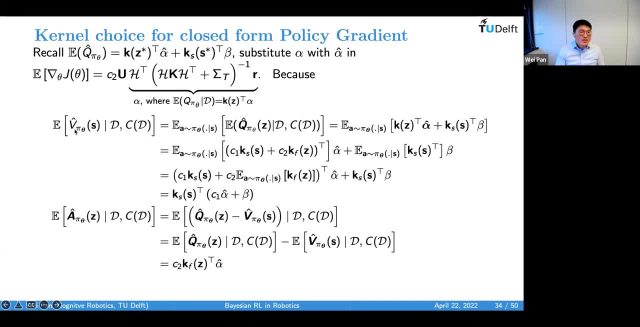 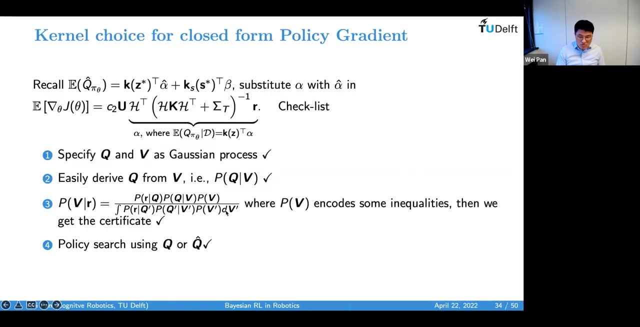 then we can derive the V hat, conditional on this data side, and the constraint side as follows: Then we can derive the policy gradient by simply using this quantity here, By using this quantity here as follows: Okay, So now we have the policy search using Q or this new Q hat. 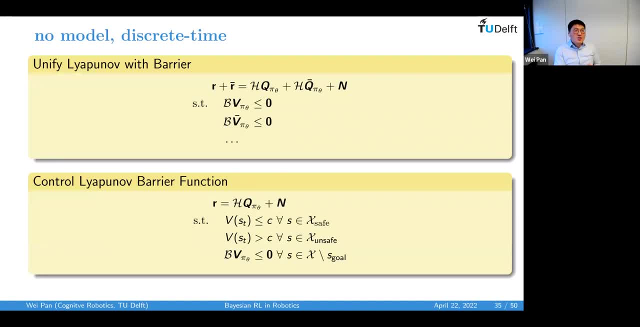 And of course, we can also unify the layer funnel with the barrier function as well. For example, if you consider both cases, we can specify two value functions and two state action value functions as well. So this V is responsible for the layer funnel function. 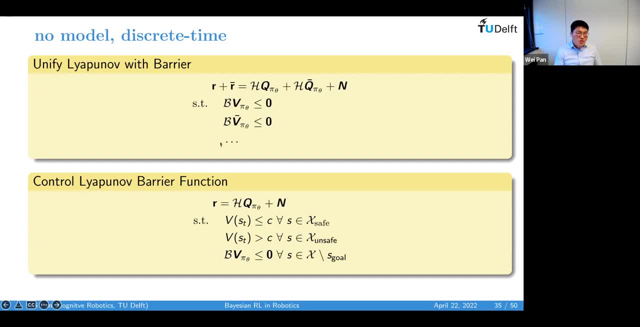 and this V hat is responsible for the barrier function. Of course you can add some additional constraints as shown in the certificate, And then also we can have the control layer funnel barrier function, which is as follows: by adding such constraints in the certificate, 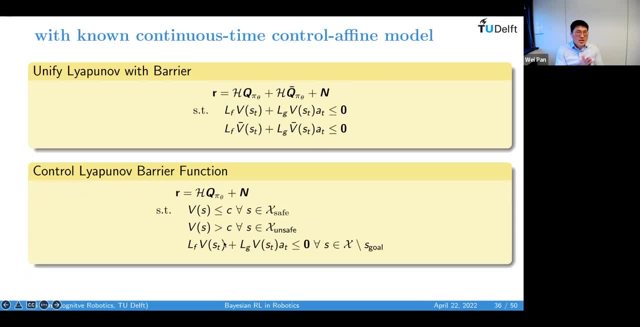 And simply, if we are given the model, that's a good idea right? There's a good news that, for example, if the system is a control of fine form, we can also add these constraints, including the model information as follows, to solve the constraint regression problem: 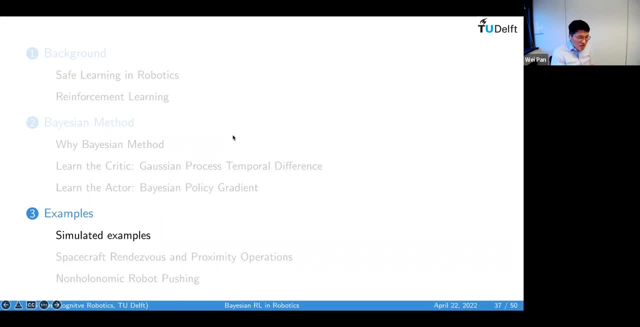 Okay, So far I have introduced the theoretical result, We have introduced the algorithms, We have introduced how we're going to solve this constraint regression problem. by using the Gaussian process And if, luckily, we get a V, V is our certificate And also we can combine. 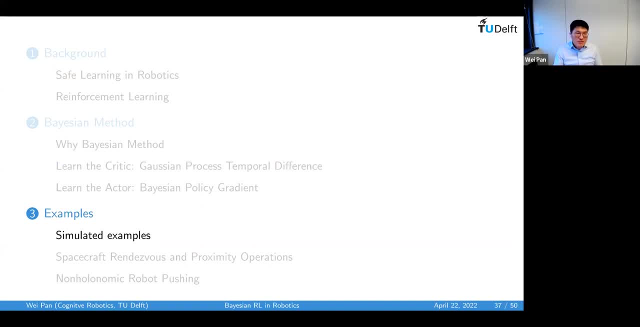 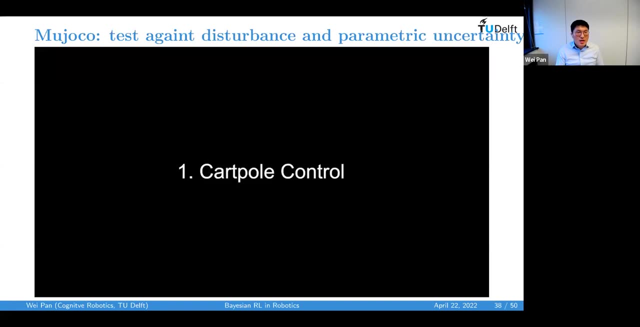 with the barrier function, et cetera, to get even more certificates. Okay, Let's see how it works in the practice. The first of all, I'm going to show some simulation examples, including the couple control, So we test against the disturbances. 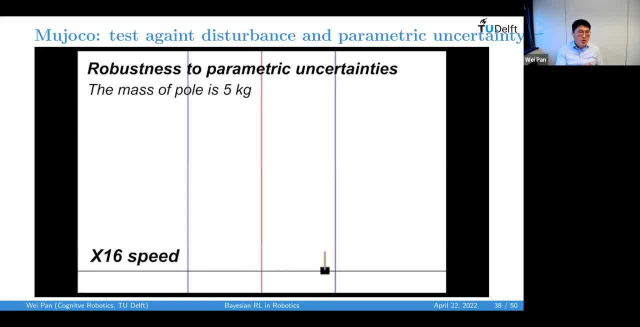 and the parametric uncertainties. We vary the mass of the pole as follows: We test the robustness to parametric uncertainties And furthermore, we change the disturbance torque to test the robustness to disturbances. In the second example we consider Hopper control. 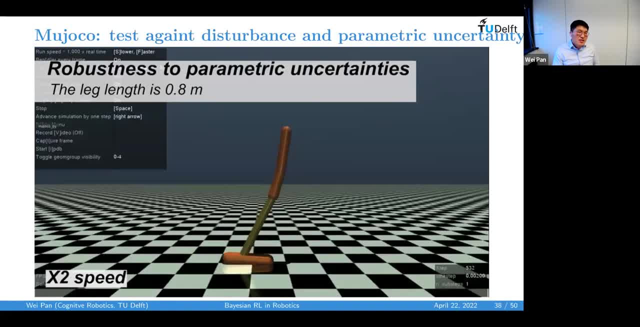 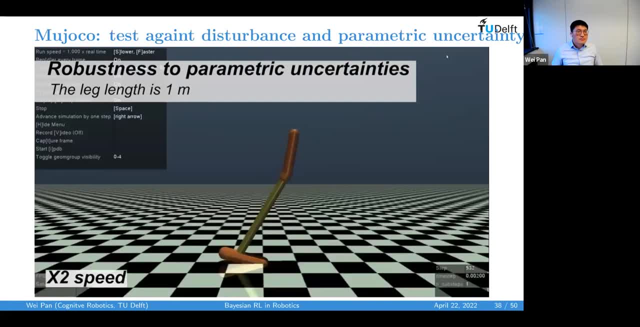 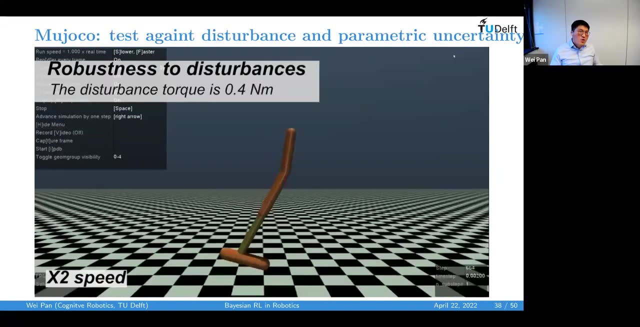 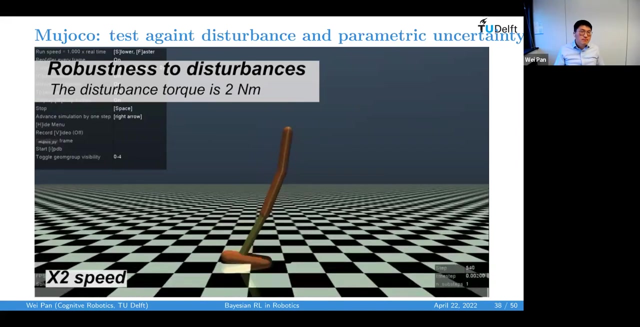 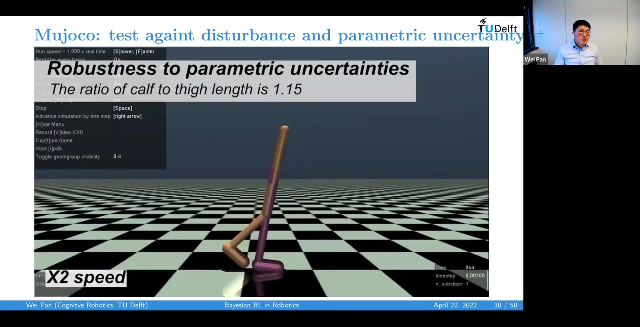 and we change the light lines to test the robustness against the parametric uncertainties And furthermore we verify the disturbance torque to test the robustness to disturbances. We also consider Walker control. So we change the ratio of the calf to thigh length and to test the robustness. 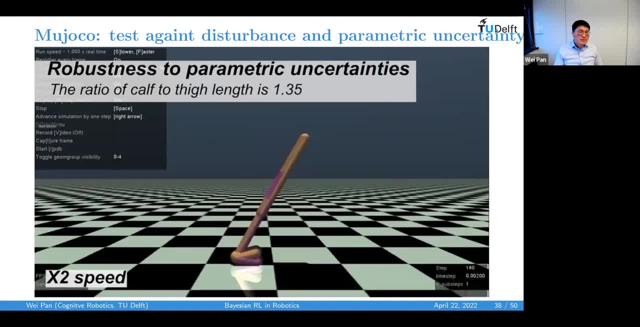 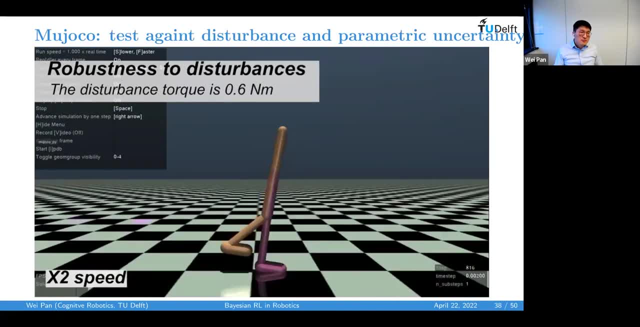 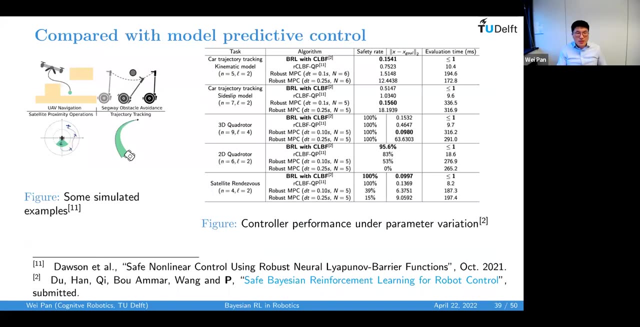 to parametric uncertainties And we change the disturbance torque to test the robustness to disturbances. Okay, We also compare with model predictive control And actually we find this paper is quite interesting. We introduce or combine the control layout of the barrier function. 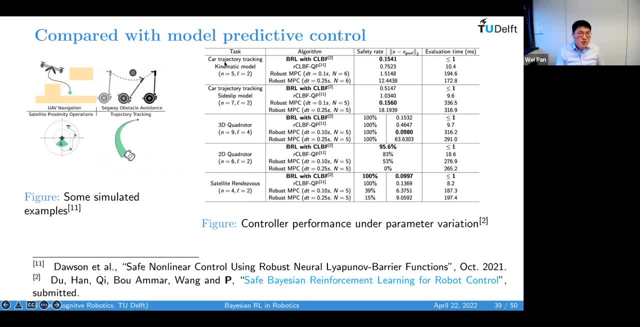 And in some similar examples like a car tracking, a car trajectory tracking with a kinematic model and a car trajectory tracking with a slight-slip model, and also 3D quadrature hover, a 2D quadrature with collision avoidance and a satellite rendezvous. 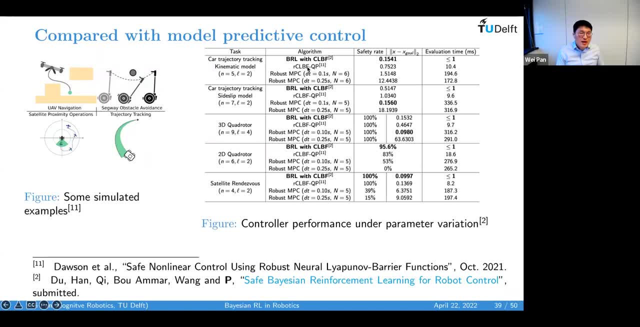 And our method compared with this method and also tested against the robust MPC method, So we can not only achieve very good safety rate and also control performance. So if you think about, okay, this kind of constrained control problem right. So I think the first thing 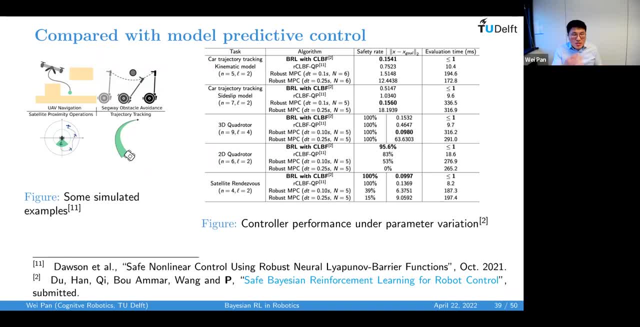 came up into my mind is model predictive control right. So we're trying to minimize or optimize some of the cost in a finite horizon, with some constraints regarding the dynamics of the model, or some constraint on the state and some constraint on action and some initial state. 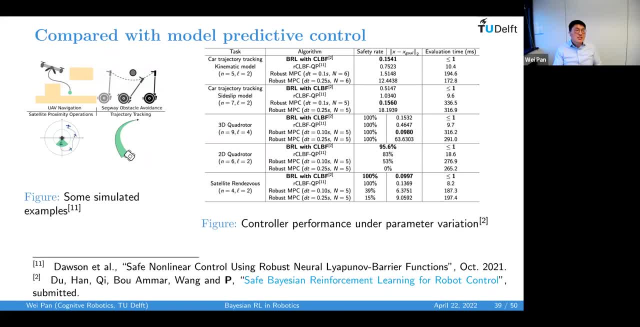 and some terminal state, And then we can solve the constraint problem easily and by using some efficient algorithms like a convex optimization and so on and so forth. right, But however, in the practice model, predictive control has some problems. For example, there's no guarantee. 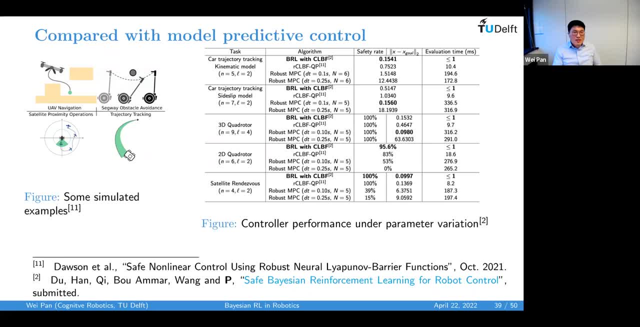 on the safety and stability beyond the linear case and the model cannot be too complicated and the constraint cannot be too complicated and the model uncertainty cannot be too complicated and also computational, too expensive for high control frequency. So this is what the result shows. So if you increase, 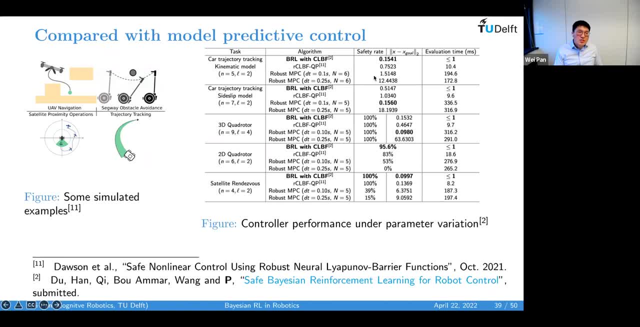 the sampling rate right. So increasing the sampling rate, the performance increases. So basically, if the control frequency is low, it's okay, but the one is high. So basically the result is not that good, And for our method 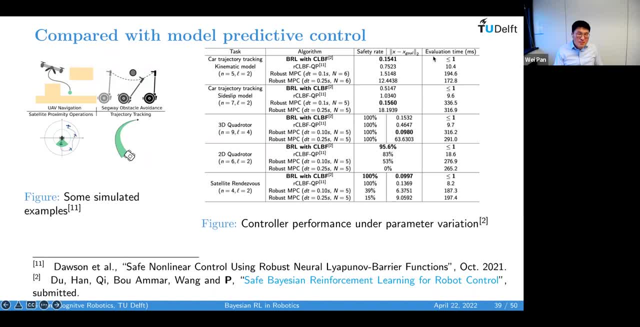 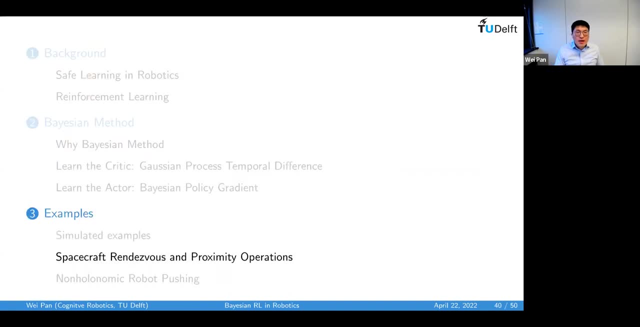 the most important thing is that I think that evaluation time is negligible because we are using a deep neural network as a policy and as a controller and we don't have to solve the online optimization which needs a lot of extensive computation. And also we show 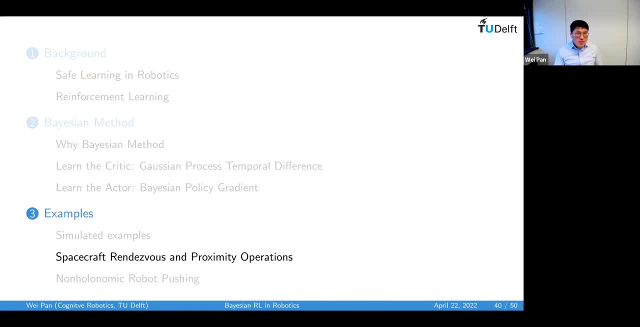 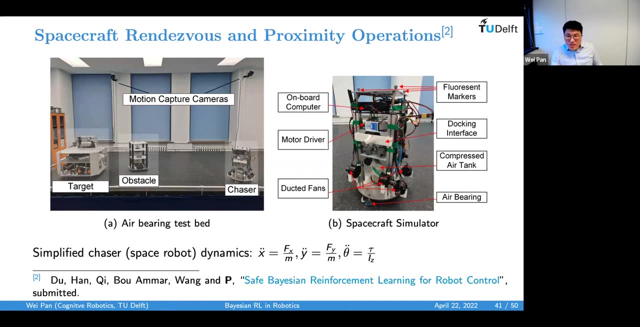 we're going to show two real world examples. So the first example is a spacecraft rendezvous and proximity operations, and autonomous rendezvous and proximity operations, as well as autonomous docking, are listed as critical technologies needed to pursue a variety of future space missions, And we are using 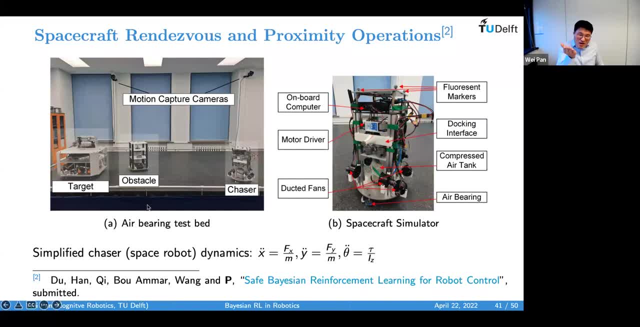 an air bearing test bag to actually to push air from bottom up to lift the robot, to compensate the gravity, to mimic the floating environment in the space. And, regarding the spacecraft, it consists of onboard computer, which is basically do the deep neural networks inference and have the motor drive. 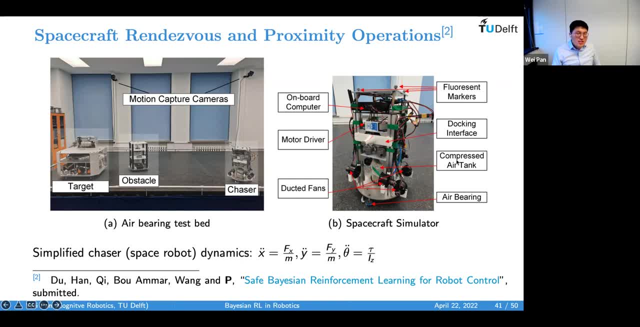 and duct the funds and the compressed air tank. So these two things are actually the actuator, So they push the air, okay, and to generate the force to move the spacecraft forward and turning around, And this is a docking interface. So the goal is that. 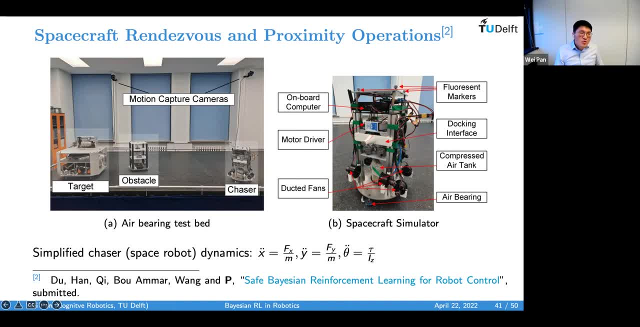 this docking phase can go through this area without collision with this obstacle and the docking with this target successfully. And since we don't consider the perception side, so we are using the fluorescence markers and the motion capture system for the localization, Well, the dynamics of the spacecraft. 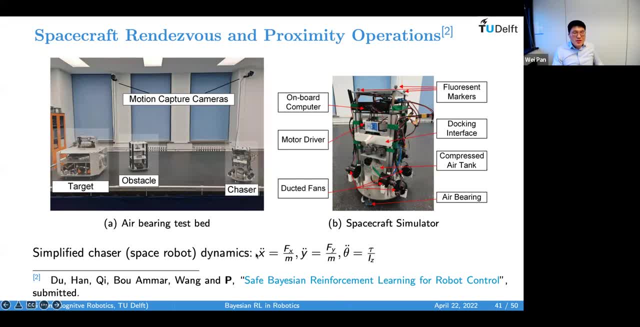 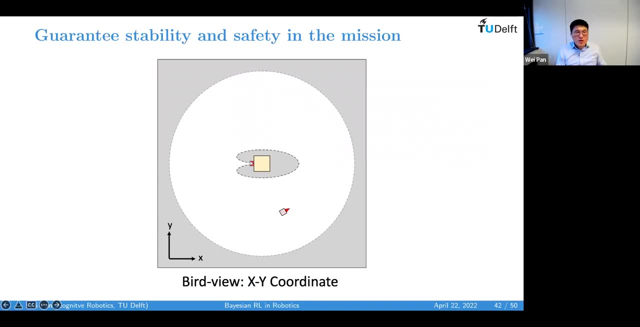 is actually super, super simple. It's nothing but a second order linear dynamics, and the X, Y are the position and the theta is the angle. Okay, And actually this task can be stated as follows: Well, the gray areas are called a key power zone. 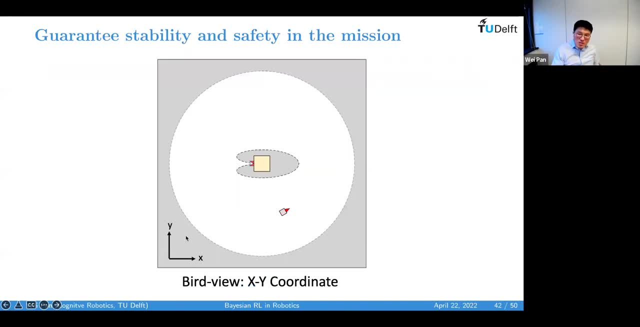 So it is unsafe. The spacecraft should never get into this area. Well, the white area is safe, So the spacecraft can adjust its orientation, speed, position and move slowly, And if there's an obstacle, it also tries to avoid the obstacle. 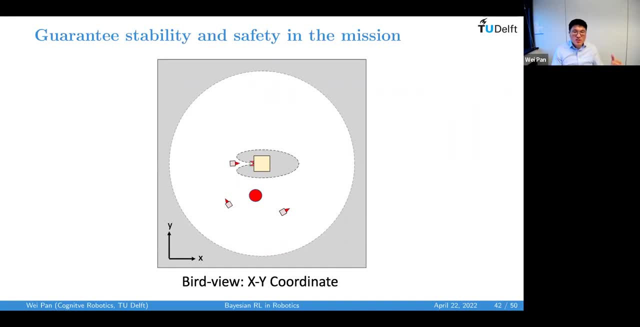 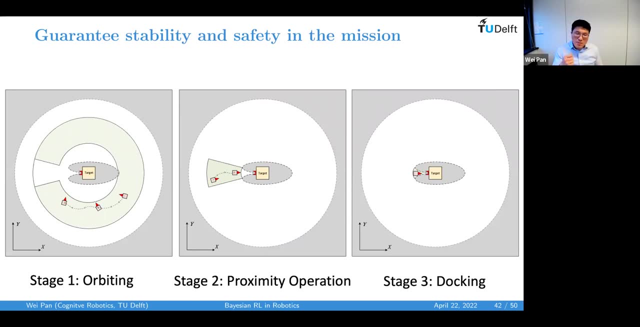 and finally successfully talk with the target. Since the dynamics of the robot are so simple, it seems that it is not difficult to complete the mission, As we also consider with MPC, right in the simulated satellite task. it seems pretty straightforward, For example, 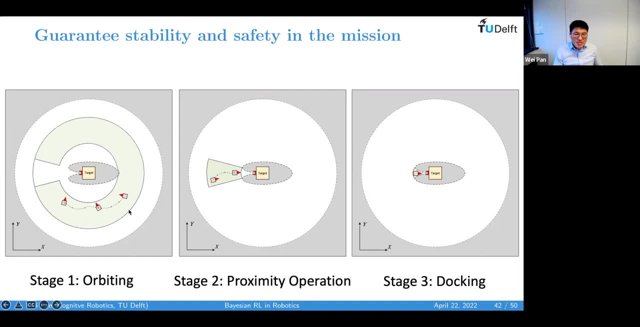 if you just use MPC, But in the practice it's not easy. The mission has several stages and some weird constraints to satisfy. The first stage is called operating. The spacecraft adjusted the orientation to get into the docking cone. Okay, The green area here. 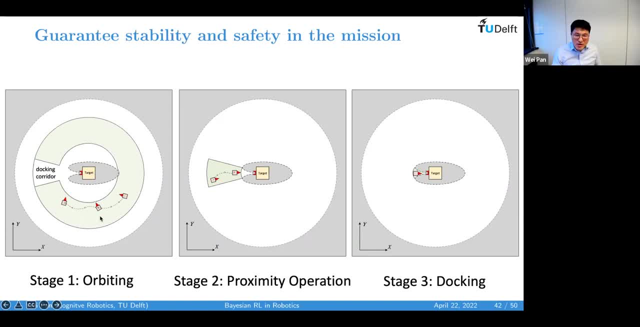 or the colored area. here is the operation area where the spacecraft is expected to stay during this stage. It can get into the white area for some reasons or for some disturbances, but also it has the ability to come back to this green area. Well, 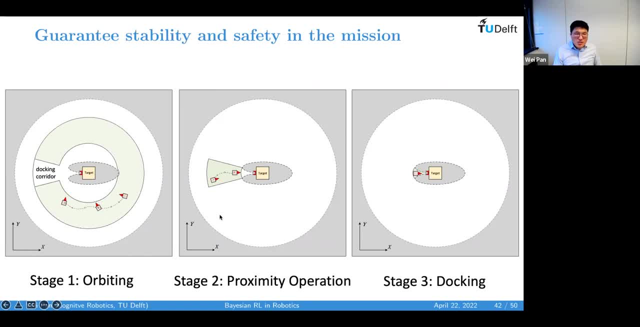 the second stage is proximity operations. So, in this docking corridor, okay, this colored area, the docking interface, okay, this arrow here should adjust to be vertical to the target. Well, on the third stage, okay, let's zoom in a little bit. 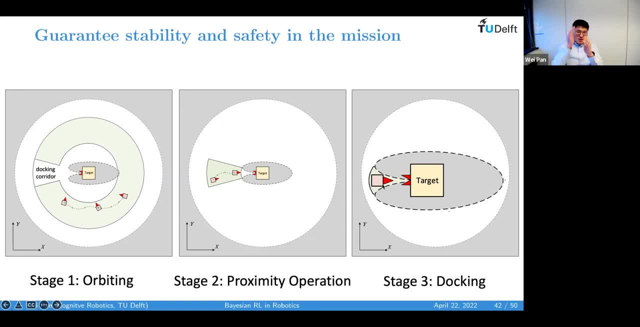 And this spacecraft should move slowly, preferably in a straight line, to dock with the target. Well, the green area here is the operation area, but it has to avoid the obstacles defined by this key power zone with this dashed line, If you see that. 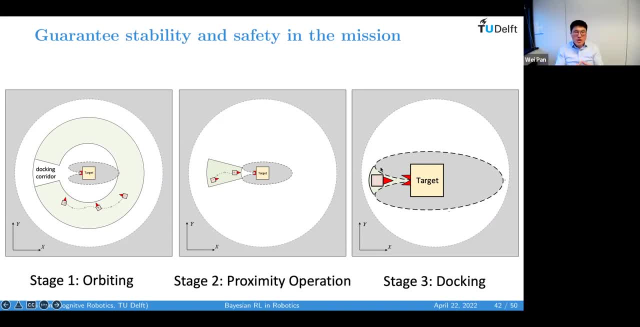 actually the constraint side of the key power zone is very weird. It's like a heart shape, right? So if you notice that, mathematically it's non-convex. So that's why model predictive control can hardly deal with such constraints. 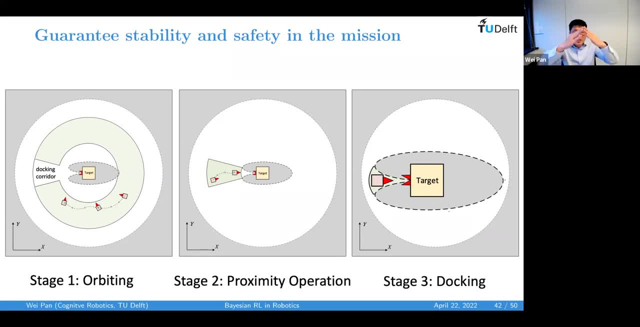 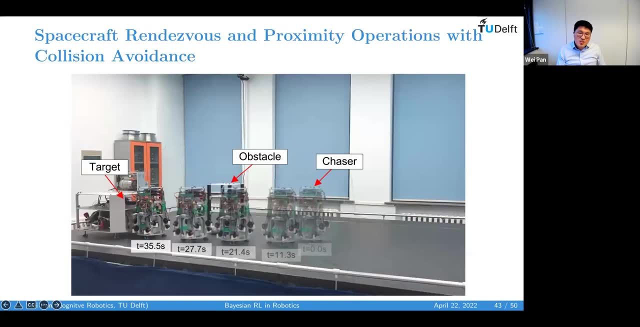 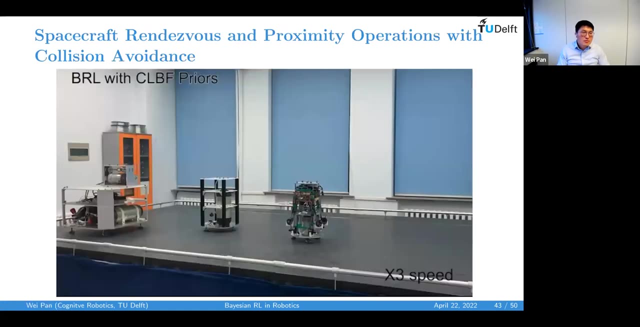 And if the simulated example, actually the constraint here, is just a triangle, so it's convex, So the MPC can solve that efficiently. Okay, let me show a video, see how it works in practice and compare with other methods. So we are using. 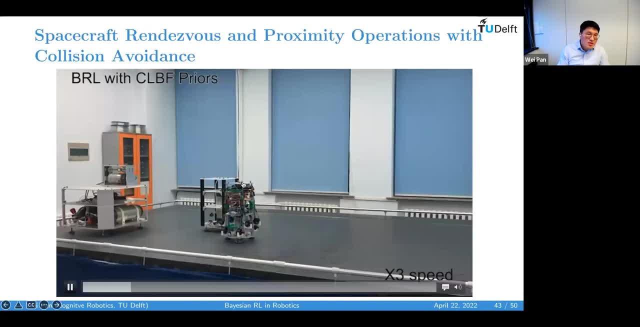 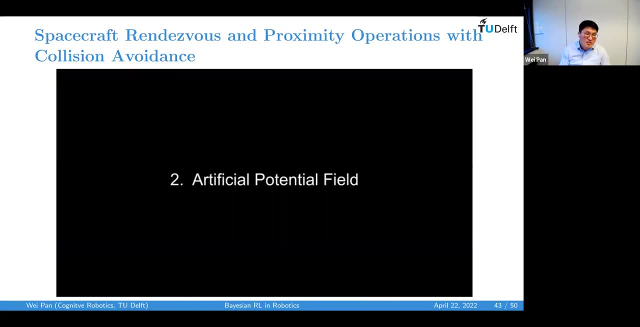 the control function as a prior, and this is the obstacle. So, as I showed, this is moved very slow And finally it successfully docked with the target And it also will compare with some state of art artificial potential field which is widely used. 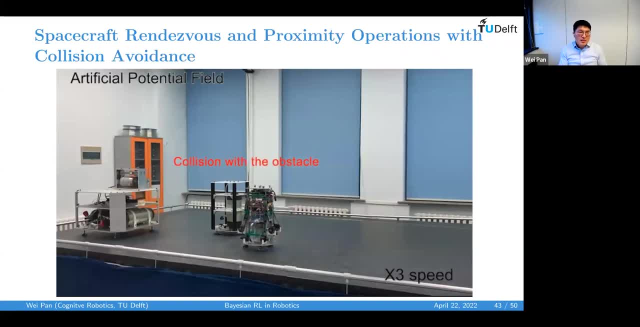 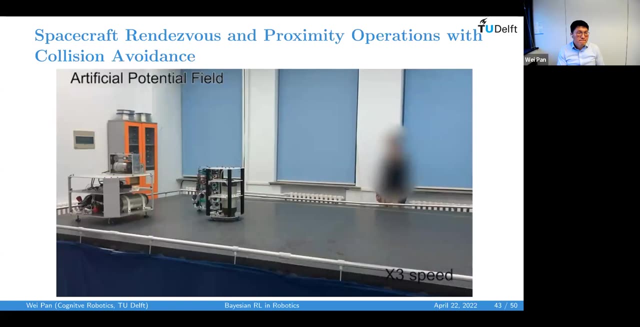 for the spacecraft, the rendezvous and docking and the collision with the. it can collide with the obstacle And also one key problem with the artificial potential field is it can also stay at the local minimum. Let's try it again. It's stuck at the local minimum. 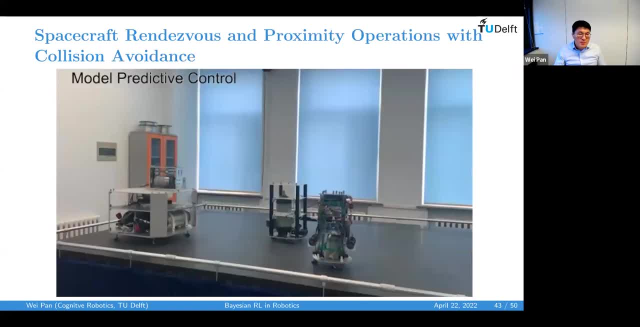 And also we compare with a model for control and see what happens. So at the very beginning the system crashed. So the problem analysis. I think the problem is that, okay, the control frequency is too high to compensate the heavy computational complex. 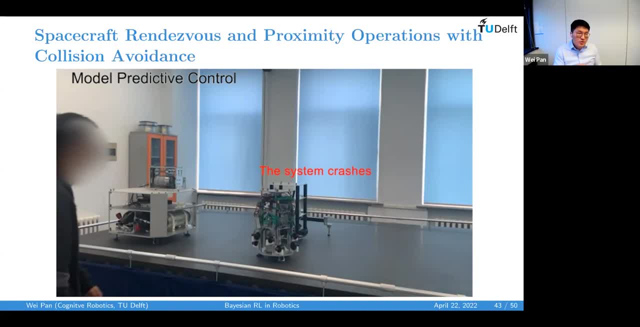 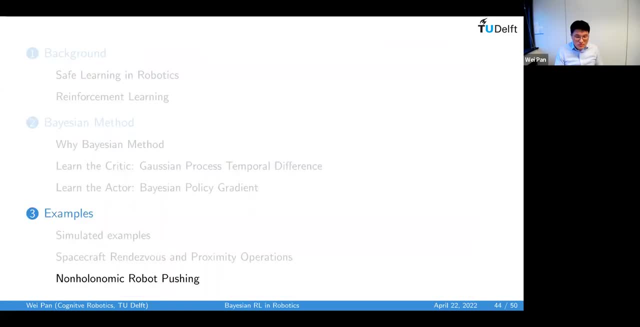 the heavy competition regarding reduced from the model for control. Okay, So I want to show one more example which is non-holonomic, non-holonomic: robot pushing. So why I show this example? because I want to emphasize the importance of modeling. 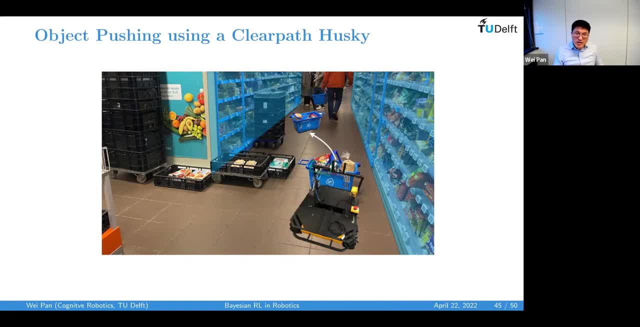 the constraints. Well, if the robot is too large or too heavy for which a manipulator or a robot arm cannot push, so we can use the UGV to push. So we consider a wheeled mobile robot operating in a flight planner environment. 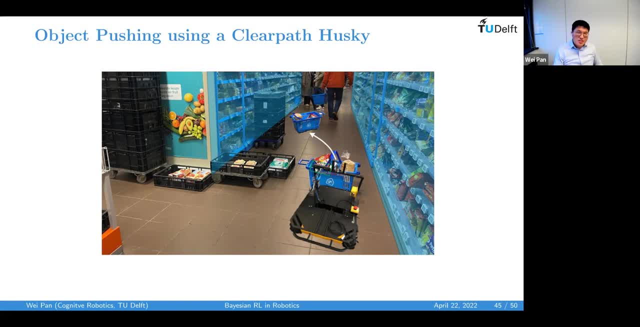 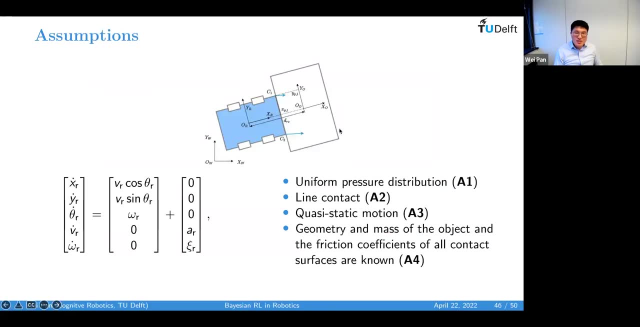 which is required to push an object to a given goal location within a given goal location. So we can use the UGV to push an object to a given goal location within a given goal location while avoiding obstacles in the environment. So typically we can write. 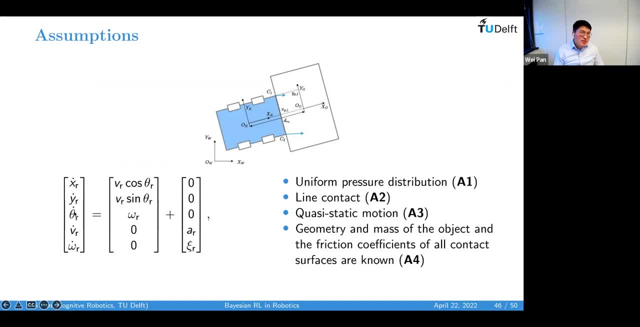 the system equation for the robot with X and Y at the position, and theta is the angle and the V is the velocity, omega is the angular velocity. so the control input is the acceleration and angular acceleration. And then we have to make some assumptions. 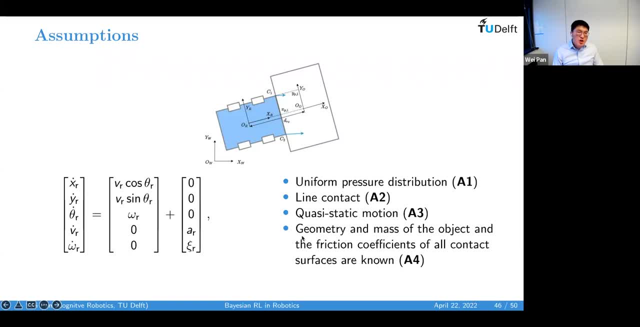 For example, unified pressure distribution, line contact, quasi-static motion, geometric and the mass of all contact surfaces are known. So basically the idea is that the object should always stick in with the robot so they can never detach with each other during the moving. 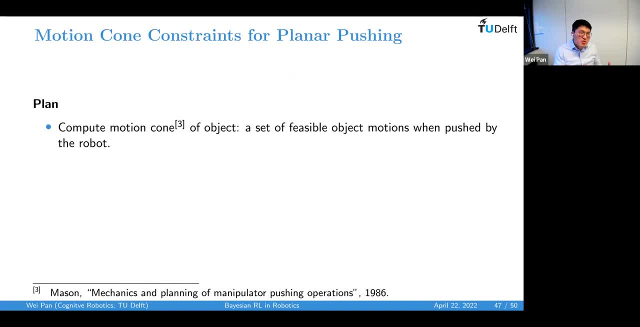 So the plan is that we want to compute the motion cone of the object, which is a set of feasible object motions when pushed by the robot, And furthermore we transform the object's motion cone to the robot's motion constraints, that is, angular velocity. 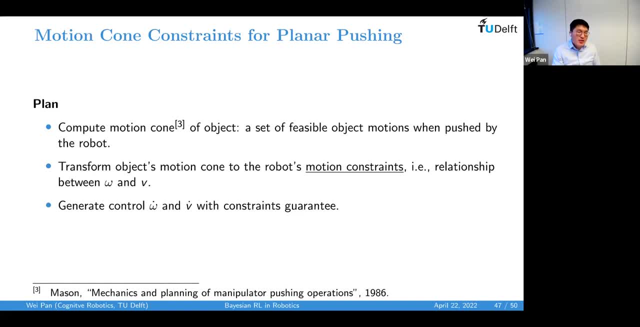 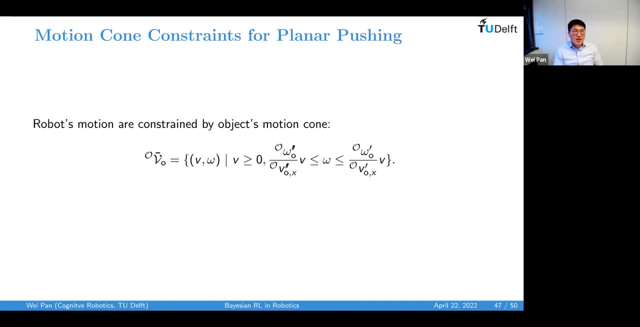 and the velocity. Then we can generate the angular acceleration and acceleration as control input with constraint guarantee. Okay, let's see how we get So by some derivations. so it's true that angular velocity and the velocity have such an inequality? 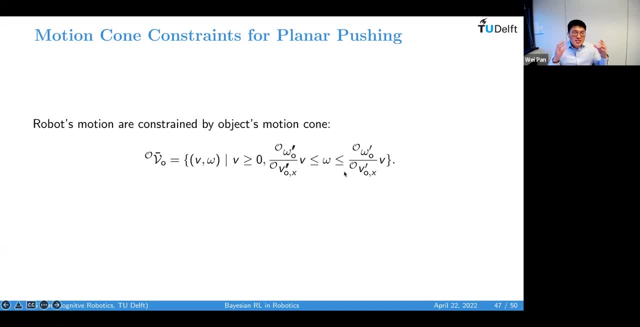 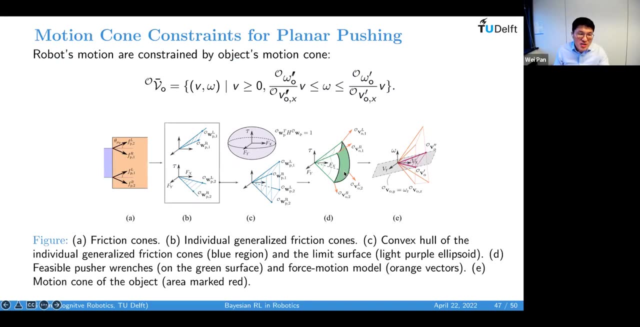 relationship and it can be used at constraint. And this capital O here is the motion cone of the object. Well, this is a difficult task, actually, because you're going to derive the friction cones: individual generative friction cones, convex hall. 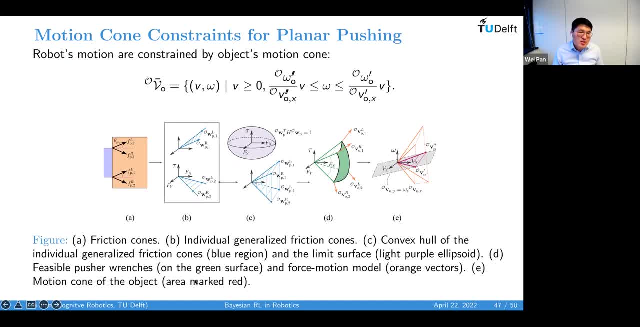 and so on and so forth, And you generate the pusher wrenches and the force motion model. Eventually we get the motion cone of the object. So what I want to show here is that, due to time limitation, probably I will not go to the details. 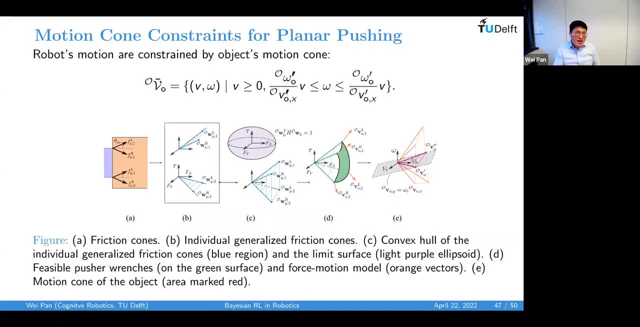 but the idea is that, okay, sometimes you have to understand the application at your hand and the assumptions will be violated, So you can get some complicated constraints and our framework can deal with complicated constraints for these situations. So let's see how it works. 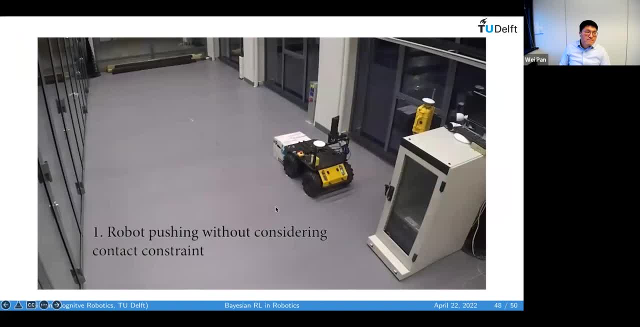 in the practice. So the robot pushing without considering the contact constraints so easily. it's just a slip away And if we consider the robot pushing with considering the contact constraint, so it can work pretty well. Now we have some more difficulty, which is the obstacle. 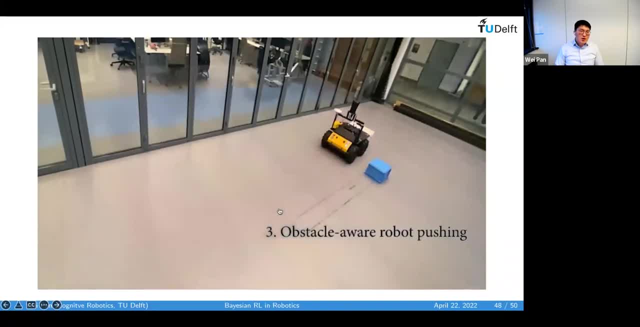 then it also can do the pushing with collision avoidance. Okay, that's it. So I introduced the Bayesian reinforcement learning for robot control and we can offer the safety certificate by constructing the value function as the optimal function, maybe some barrier function and so on. 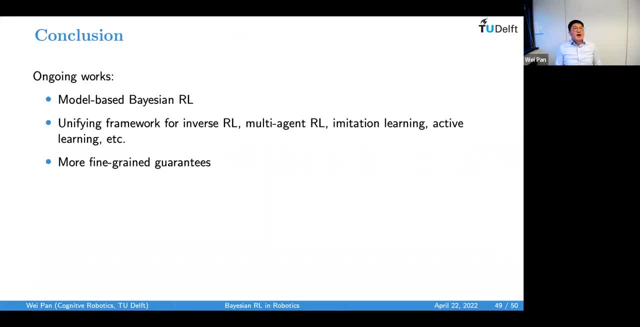 so forth, And there are actually some ongoing works I want to mention. So one is the model based on reinforcement learning. So typically we have the model based on reinforcement learning. So the model based on reinforcement learning, typically we are rarely have the mathematical model. 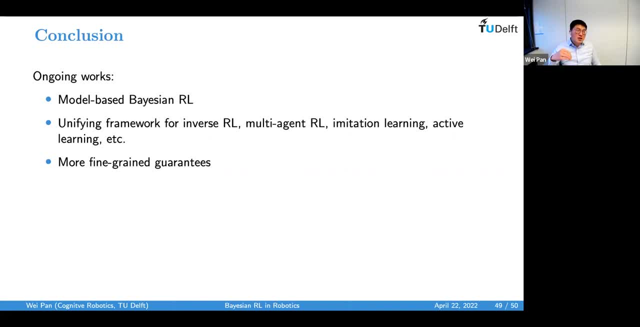 we can only try to learn the model and during the learning we are using the exploration, we are using the information of the uncertainty of the parameters to get the policy search which is more efficient And, furthermore, we want to unify these other reinforcement learning. 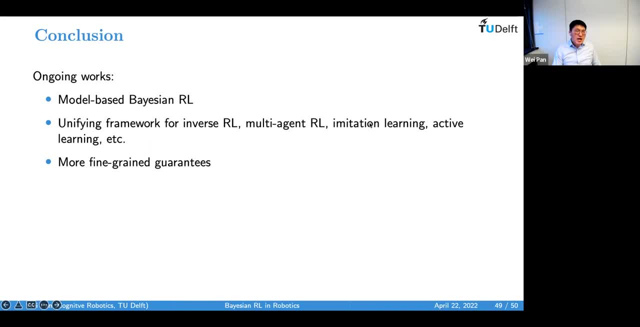 frameworks like inverse reinforcement learning, multi-agent reinforcement learning, imitation learning, learning and so on, so forth- Then if we can inject or priors on these safety certificates- and there are going to be a lot of applications for these frameworks- 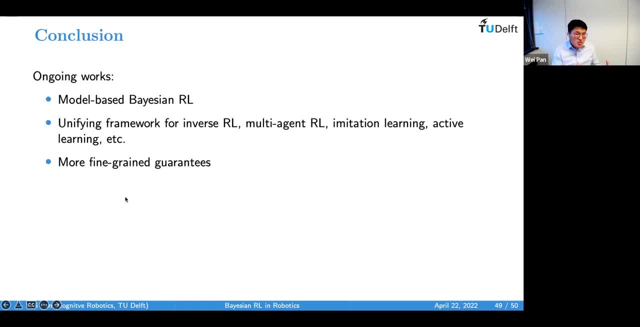 And furthermore I just gave a little bit introduction on the safety certificate. So definitely there are some further directions we can explore more on the fine-grained guarantees. However, there are some challenges, which is critical And also we mentioned a lot. 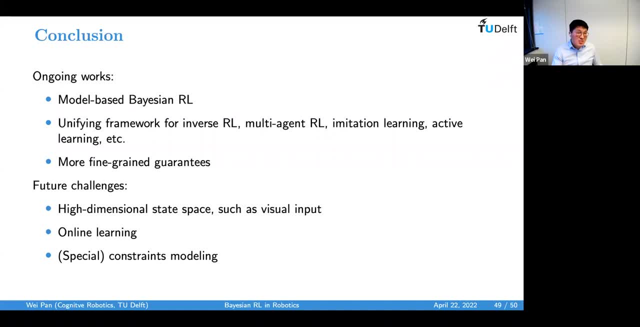 actually during the discussion with the faculties before this seminar. so one I think the most important issue or the challenge is the high-dimensional state space, such as the visual input. Now I only consider like the state of the robot, like the velocity. 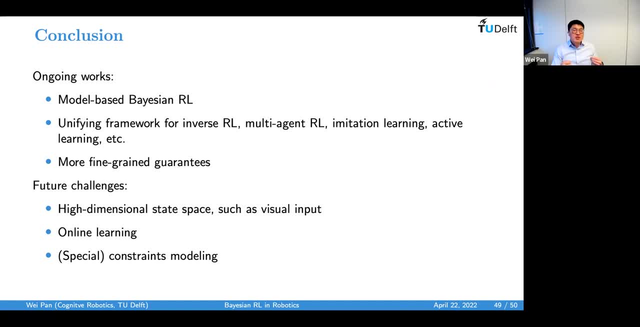 position and so on, so forth. And how about the visual input? And also, in my case, I'm using a motion capture system. So, basically, localization is not a problem. Then how to deal with the localization regarding from some sensor data? 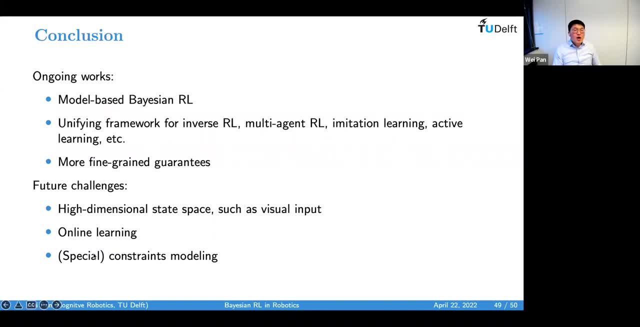 and high-dimensional data is a problem And, furthermore, we are doing the offline learning. okay, How about online learning, like in the model project? control in the dynamic environment And, of course, the last thing is the constraint modeling for the application at hand. 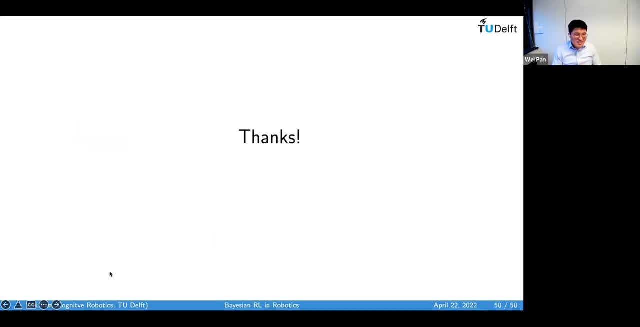 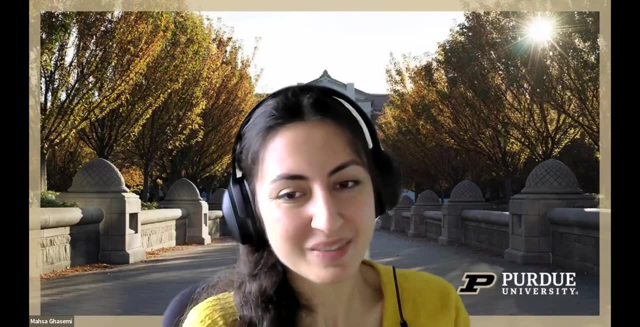 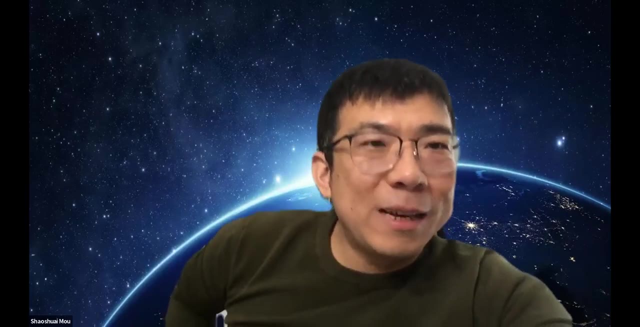 and for your particular interest. Okay, that's all, Thank you very much. Thank you very for the amazing talk. Thank you very much. Yeah, it's certainly a very great seminar. Yeah, so I think we have time for some questions. 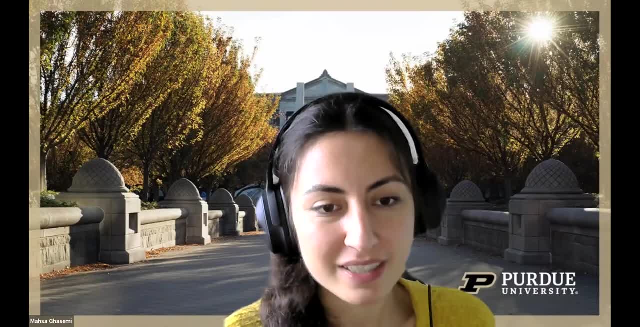 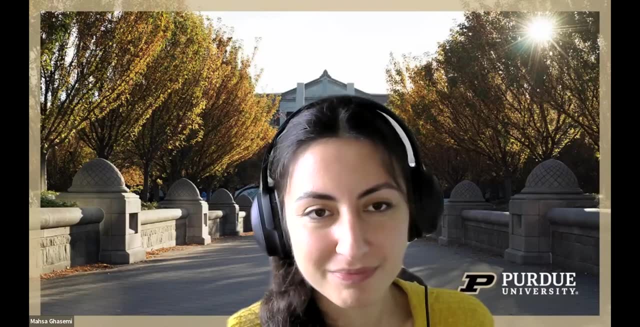 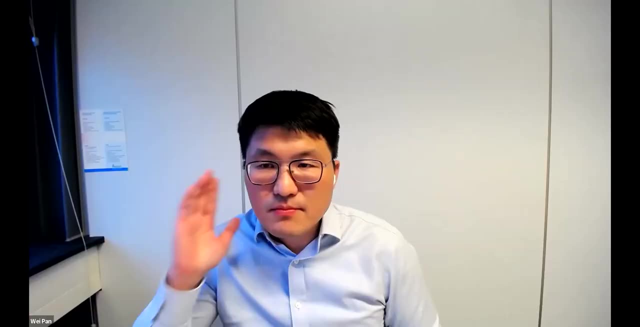 from the audience. Please feel free to either type in the chat or just unmute yourself and ask the question. Okay, maybe I can start with a question. Very nice work. So I guess one of the challenges in model-based versus model-free is kind. 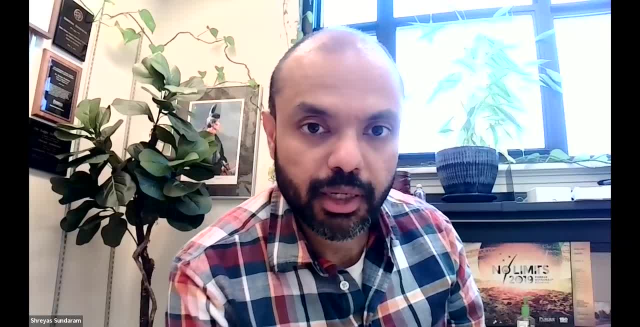 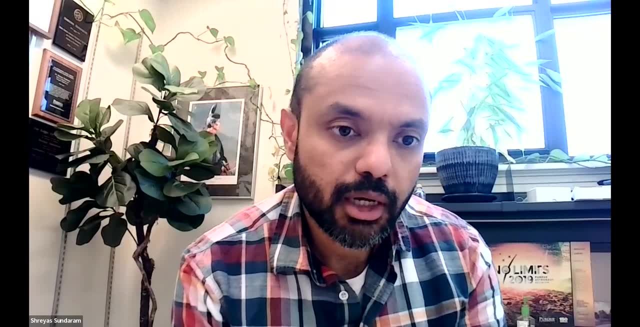 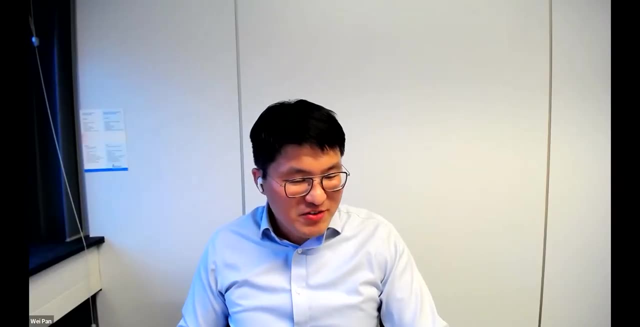 of the sample complexity right, You need to explore a lot to be able to come up with something as good as a model-based approach. So in your setup here, could you comment a little bit more on that? Yeah, this is a very 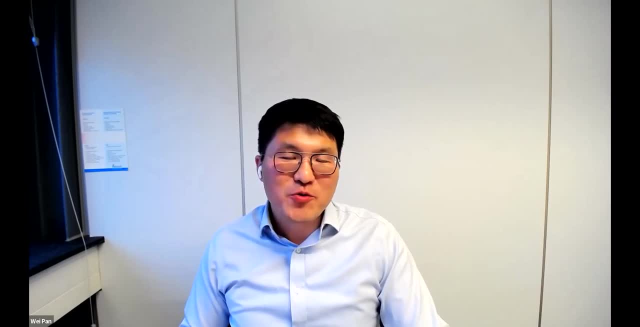 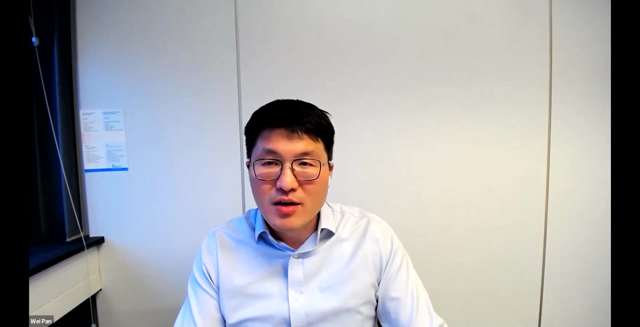 good question And actually we're kind of sneaky that we're trying to assume that, okay, we can cover all the state space and we can run all the training and run all the research that we're doing. 해요, It's an innocence. 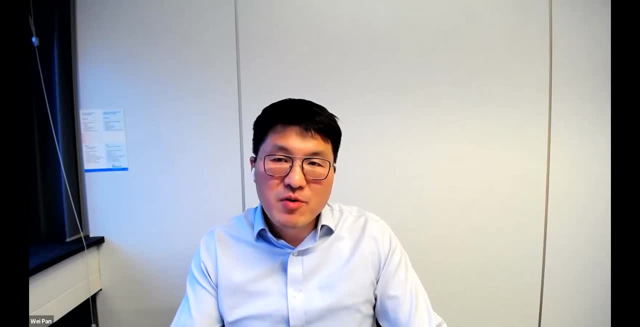 issue. To be honest, we didn't consider that, But definitely I think there are some work on the guarantee, like, okay, we can show some sample complexity regarding some performance, et cetera, et cetera, Not only for the model-based. 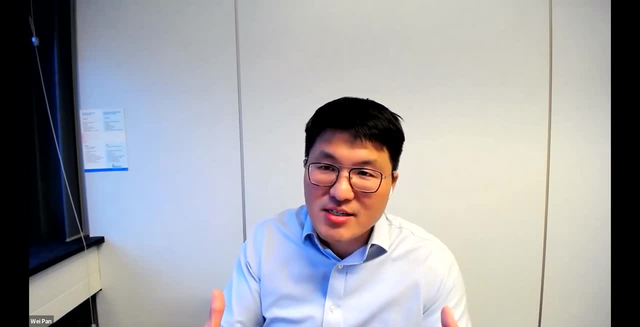 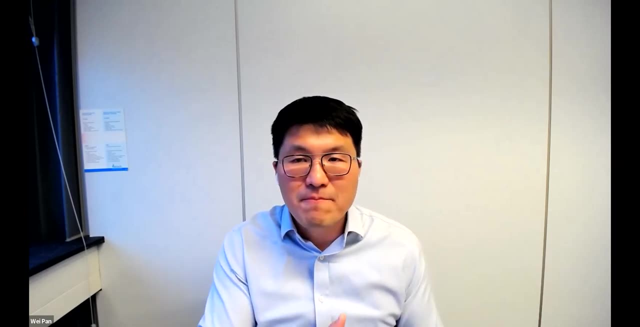 case, but also for we're going to use the Gaussian process as the policy or as the value function. So there are a lot of research in the Gaussian process community, like in the Bayesian world of the machine learning. So they're going to show the sample complexity by using some guarantee as well. So they're going to 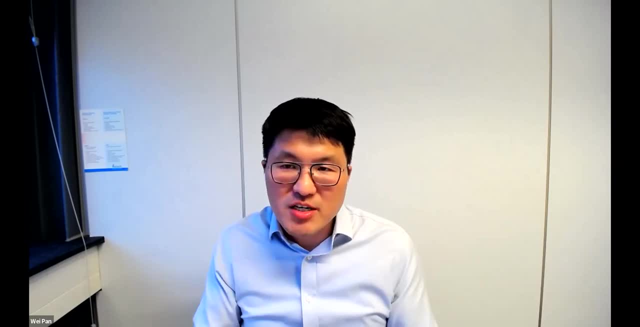 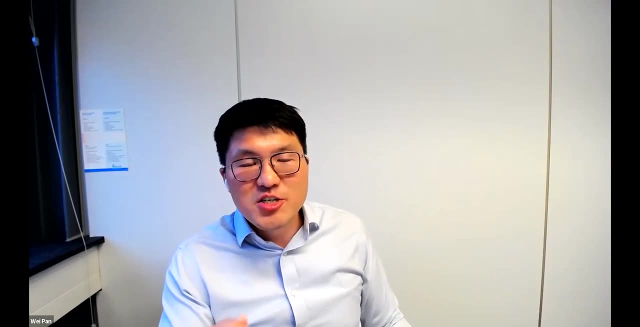 show if we have some data set and we assume some distributions, that we can guarantee that, okay, this sample complexity can be guaranteed. And the last: I think in the practice I didn't show here actually we're using verification. So verification is basically say, okay, you're. 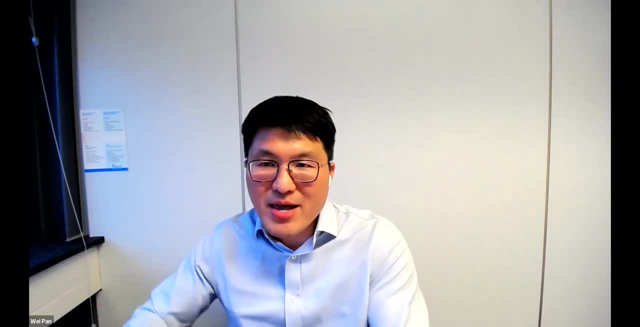 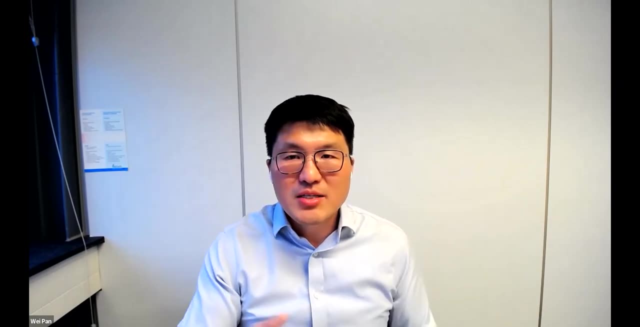 going to find some counter examples that okay, this counter example can be added to the training set to further train your neural network, or value functional policy, et cetera, et cetera. But definitely this is an important question and I think we should consider that. 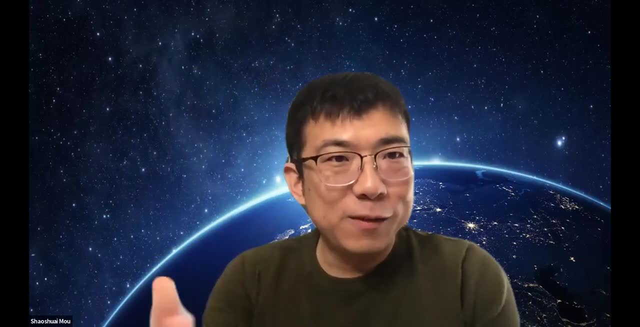 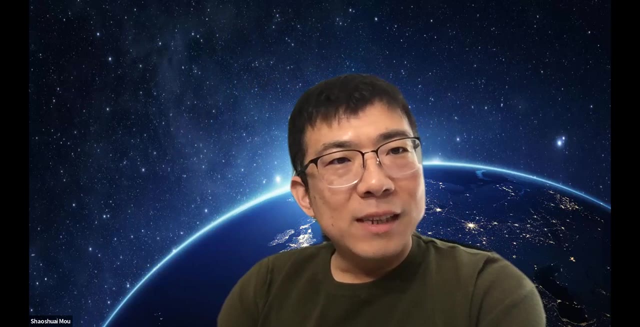 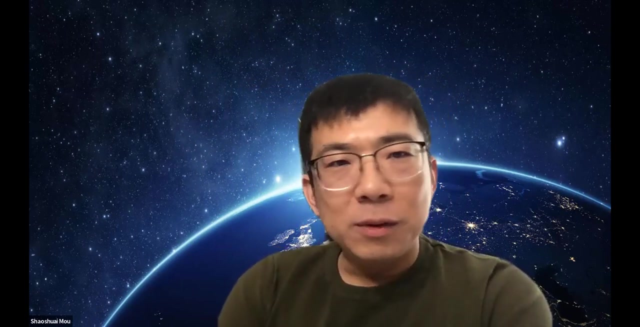 Okay, a question from me, And so thank you very much, Li, for a great seminar, Very nice, very interesting And, for you know, using Bayesian-based method definitely had a great advantage of dealing with uncertainty. So have you considered like a deep comparison between, for example, let's just 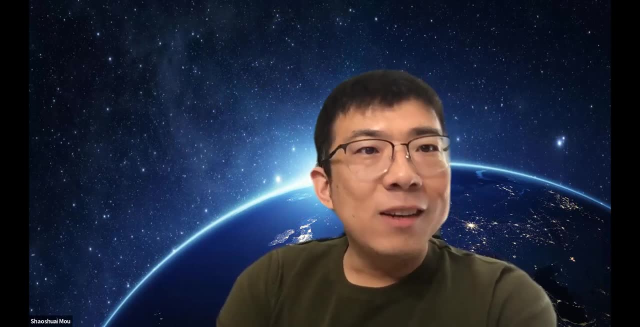 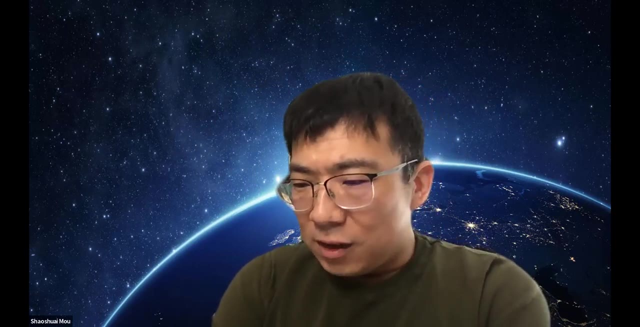 focus on data-driven model-based method, For example, giving a nonlinear system like nonlinear time-varying unknowns, and then you know you can observe everything, X and U, And then you know what is the advantage of Bayesian-based method over, for example. 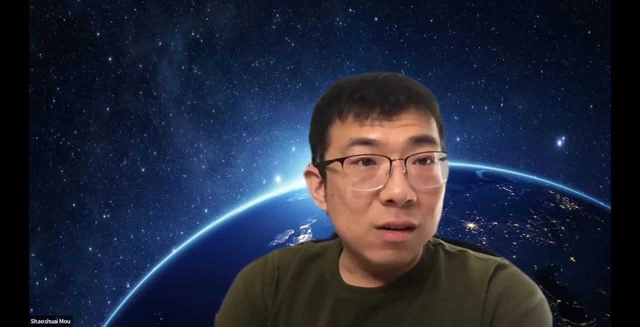 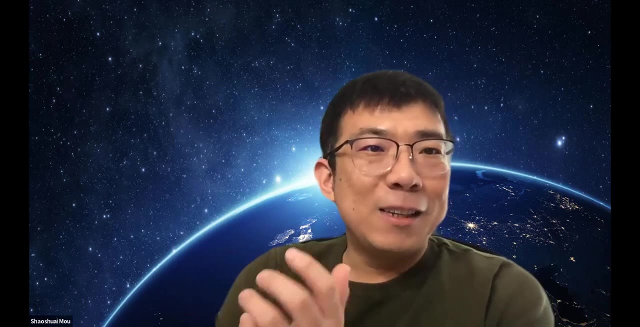 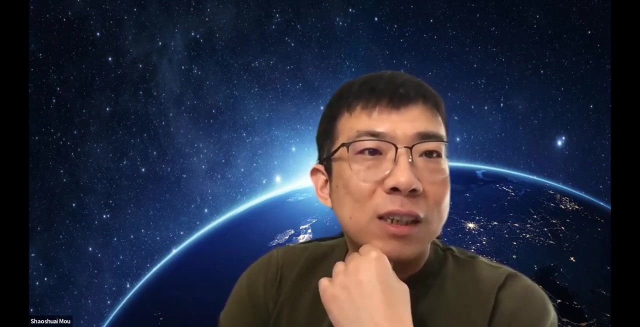 existing, like Kupman, operator-based data direction. You know, basically there's nothing, just introducing kernel-changing function, and to change the variable to be another domain, another subspace, You could use deep neural network or whatever that can nonlinear function. So do you? 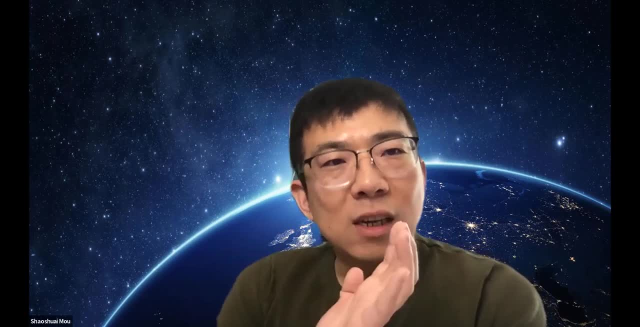 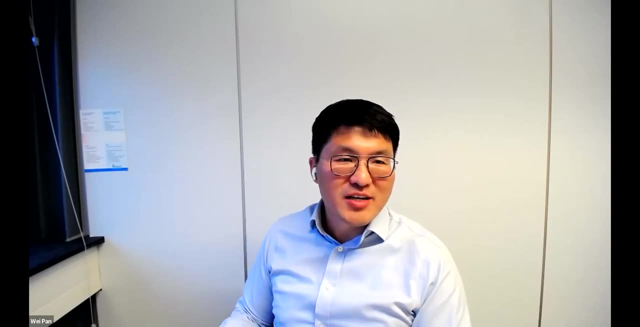 have any insight on this kind of comparison for just data-driven model-based different method? Yeah, so this is a very nice question. So actually I'm working on Kupman operator as well and Yeah, So I think I can answer this question. So, first of all, by using the Bayesian method. 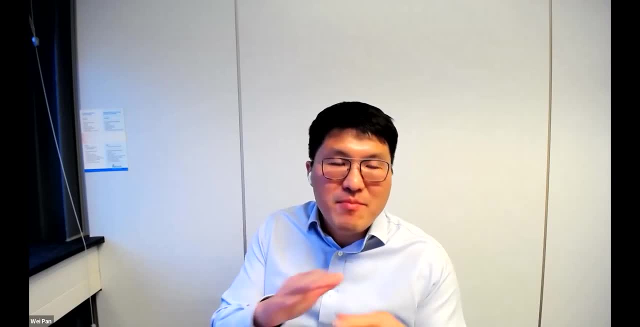 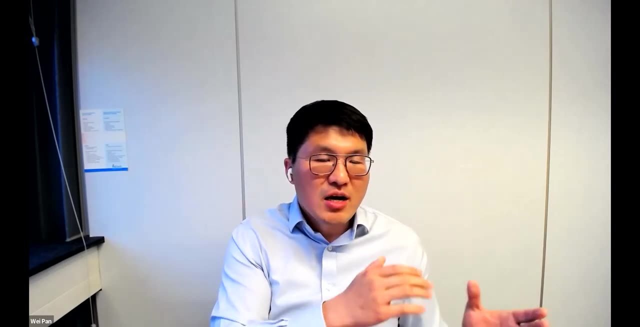 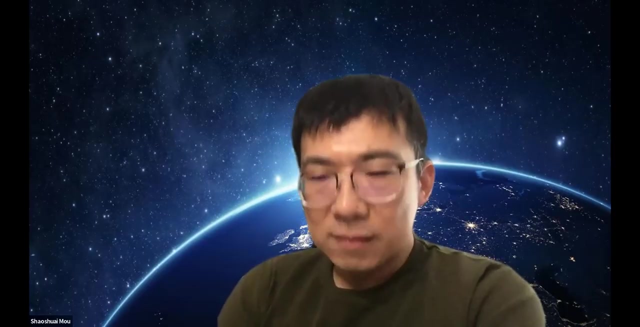 I think this is Actually this is a framework. So basically for any method or for many machine learning algorithms, you can use the Bayesian framework, basically formulated as a probabilistic interpretation of all the things. all right, So one advantage of the Bayesian method is to inject the prior. So typically okay, suppose we. 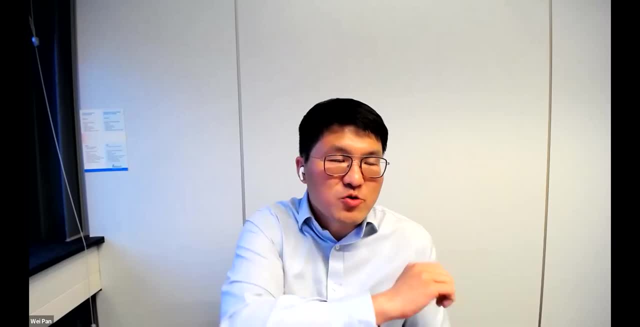 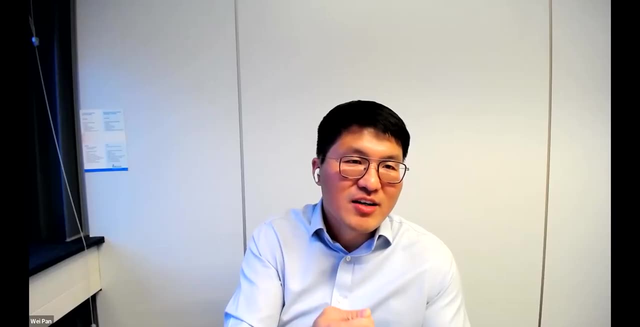 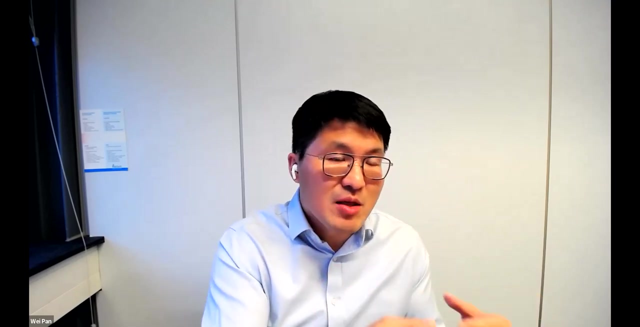 want to learn a model. by using the Newton dynamics We can derive all the F equals ma. okay, And suppose you want to learn F equals ma. So basically, you want to uncover the natural laws from data. How can you going to do that? So typically, we're going to inject some of the 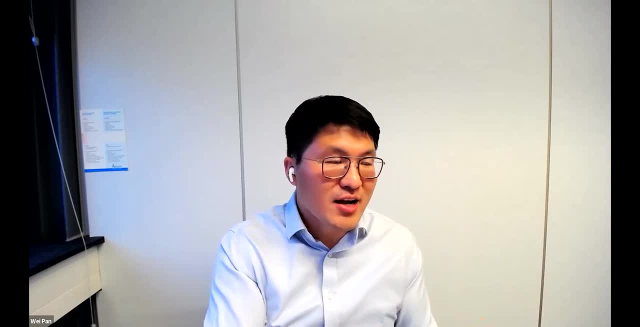 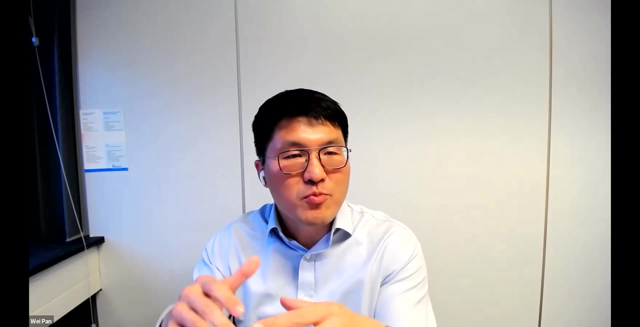 priors, Like there is a lot of work recently on the physics- you form something, something deep learning, whatever. So basically they are trying to inject the priors or prior knowledge of the physics into the modeling process. So in that way I think that's for sure, not only for scientific. 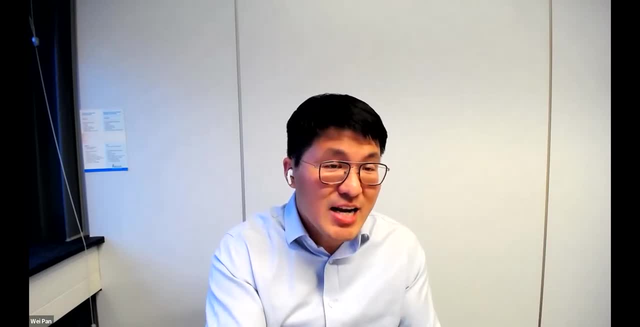 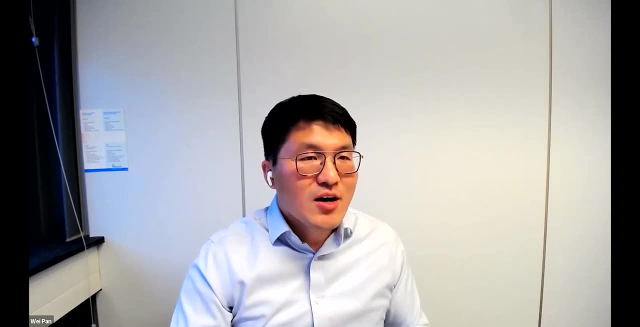 perspective that you can send. you can have some scientific discoveries, but also it is more generalizable. This is one thing, And the second advantage, I think, is that, okay, this is what we do. this is what I did before for my PhD thesis regarding system identification using sparse. 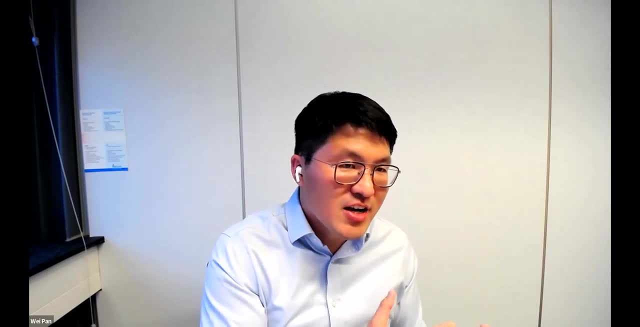 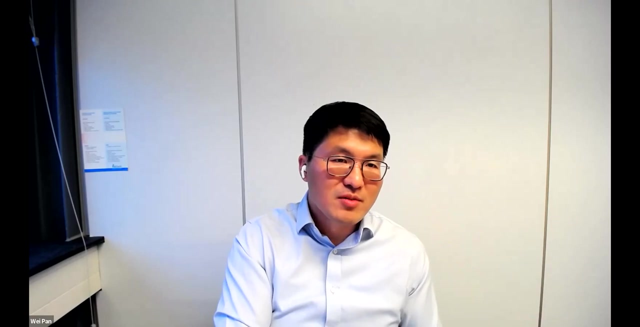 priors. So sparsity is very important in system identification And also in the Kupman operator modeling. they also use sparse in sparsity in the regularization right. So if you have a sparse model, so typically you can trade off or can avoid overfitting problem And by using 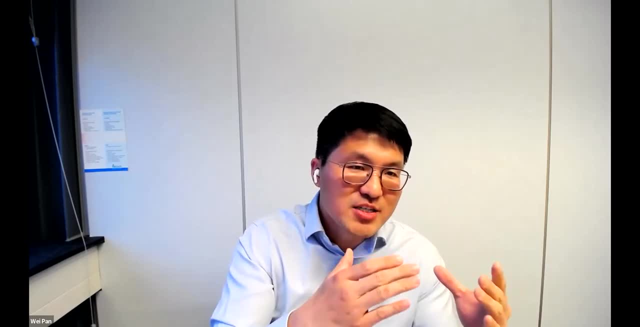 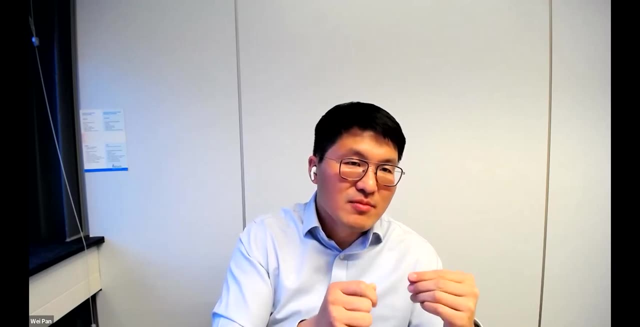 the Bayesian approach. it is a natural regularization by injecting the sparse priors, So you can get a sparse model and you can get less overfitting problem. Okay, this is the two main issues that the advantage of the Bayesian method can offer, And the third is actually you. 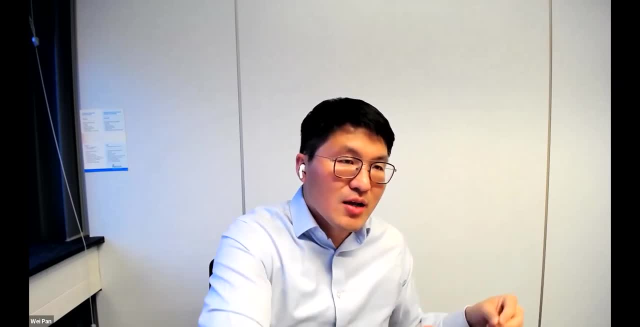 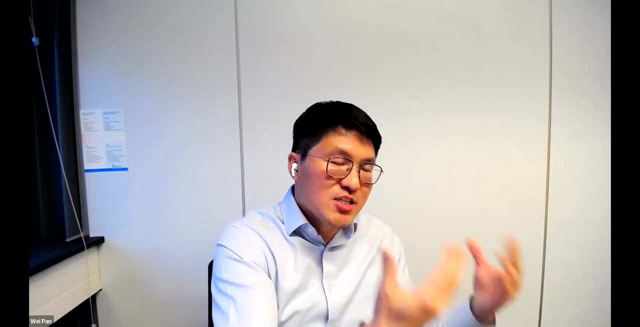 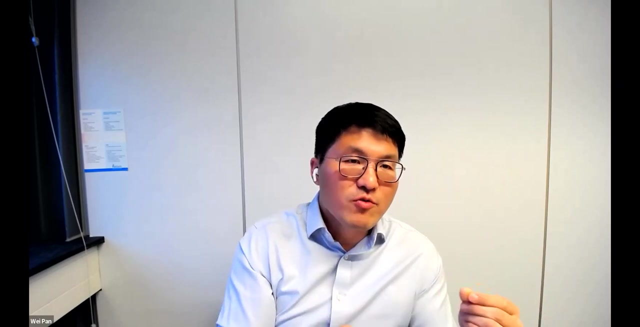 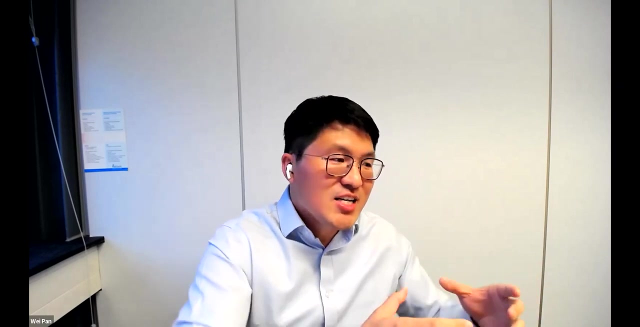 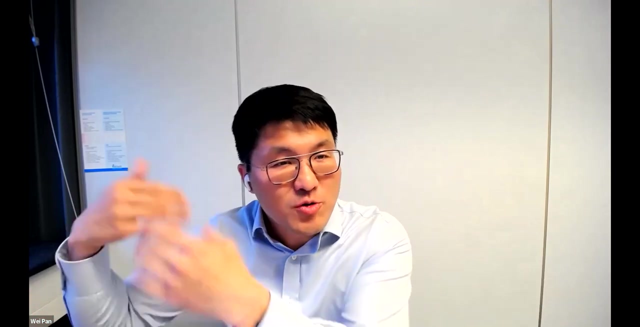 could combine the Bayesian method for the modeling with the Bayesian regression. So this is the diyex anyways, in a very well expected way of modeling the 68- protective indexing gravy pattern. this doesn't need to be without a rather icher graal in question. 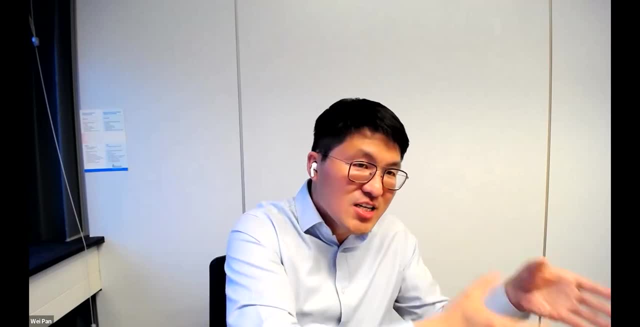 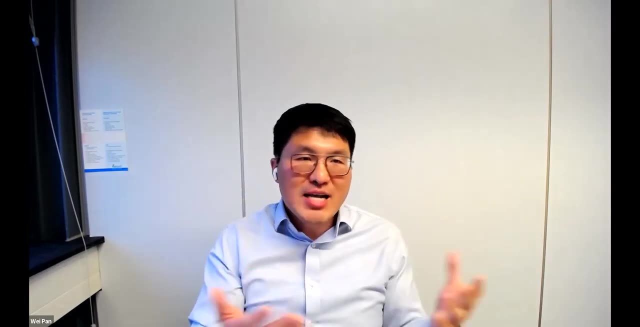 I think the work we're doing here in Washington, we're doing a basic study to document naive- they're going to update the search that you are using, the uncertainties of the parameter. so this is very nice. and at the fourth point, i actually i want to mention, if you are doing like a perception, 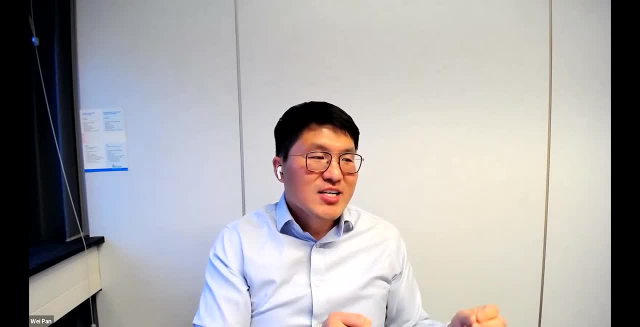 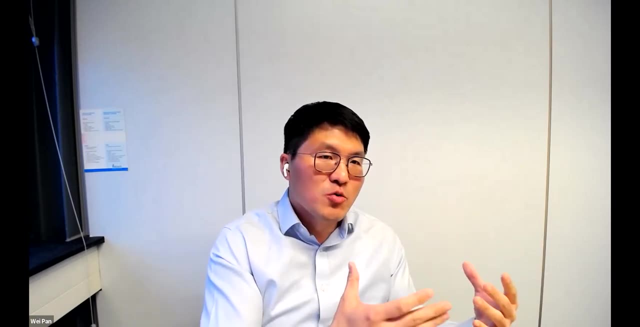 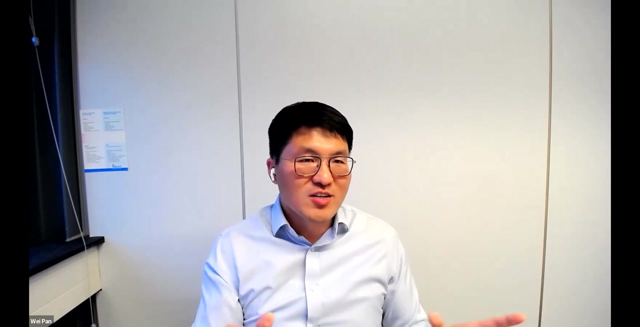 task. you want to build a neural network for computer vision- okay. so this is a basic method. actually this is from our work. we can do the basing compression- okay- of the neural network so which can be deployed in the low computational uh required platform, like as pga and so on. so far, 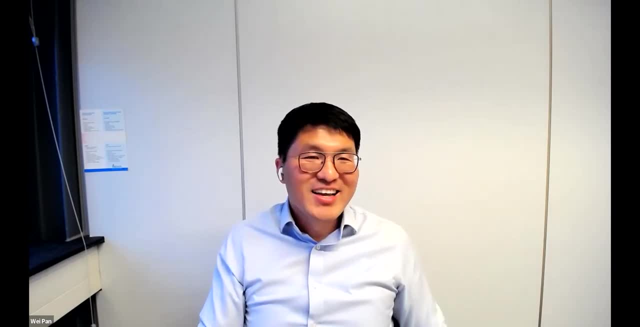 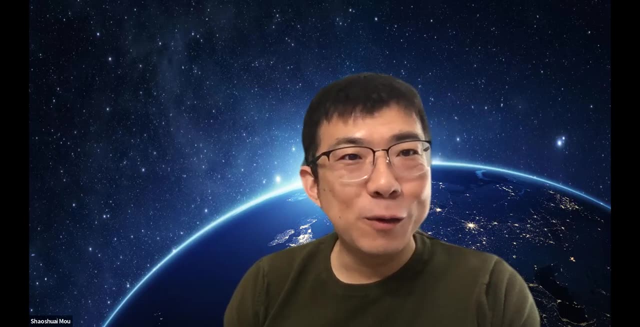 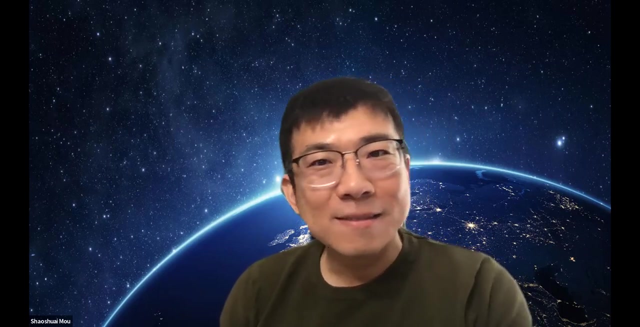 so this is something, uh, we are quite liking, or in favor of the busy learning. yeah, oh, that that's very nice, especially the last day when you mentioned- and if you got to do this compression, that you know, uh, very impressive. we're definitely follow up with you, uh, after the seminar, thank you. 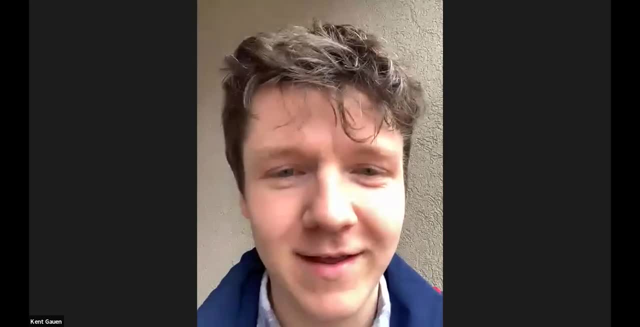 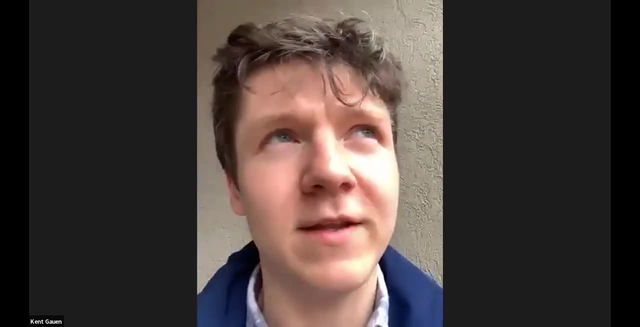 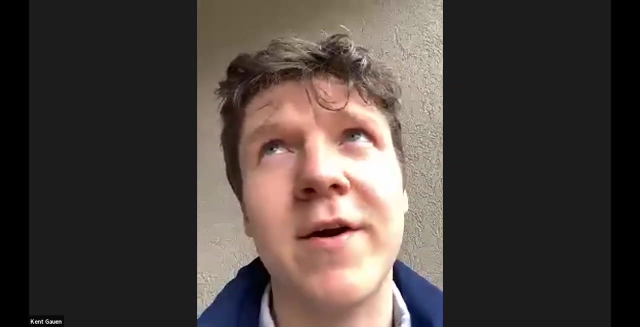 hi, dr pan, i have a question, if you can hear me okay. yes, um, i i was wondering um what the uh, how big your uh matrices were for the covariance terms in your uh example earlier. and the reason i ask is because i have a project i work on where 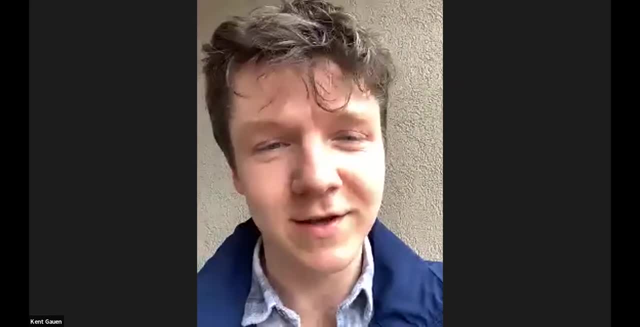 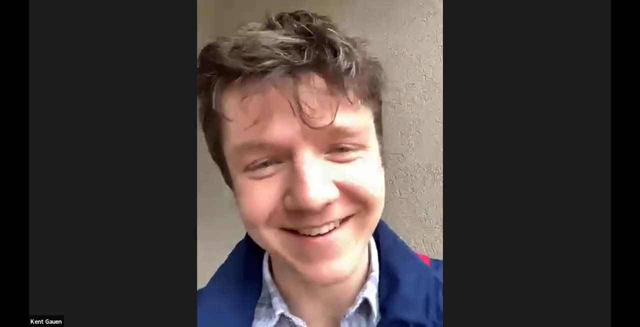 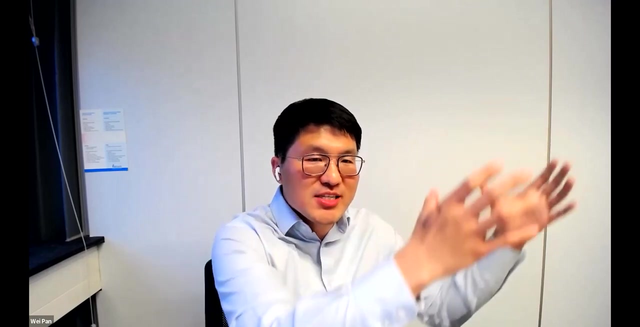 i have a reaction process with lots of tiny matrices: 20 000.. oh, 20 000. okay, yeah, that's expensive. okay, yeah, that's expensive, yeah, so basically we update i as follows: so basically, uh, we're using some initial state, we're going to sample this size. okay, once it goes on, goes on.